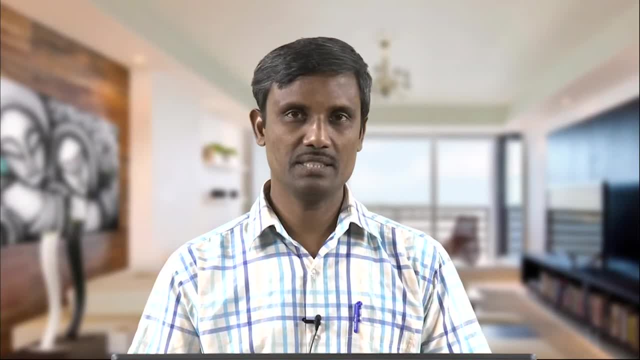 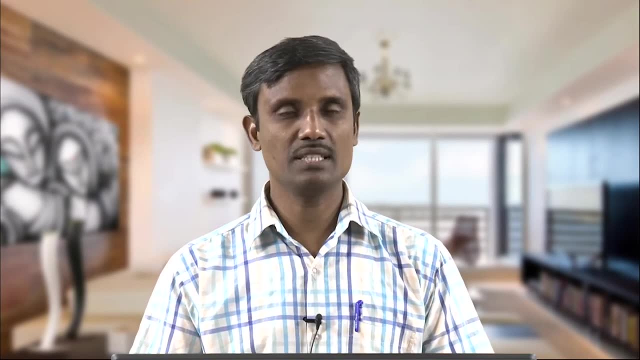 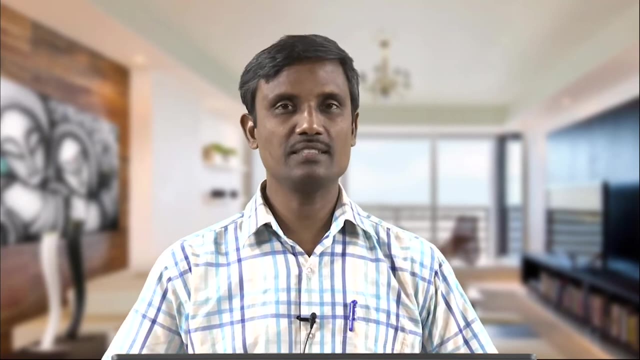 started the interaction of radiation, So the interaction of radiation with matter in the previous lecture, and I have covered interaction of charged particle with matter alright, So that comes under recap and then more about the detectors I will discuss in today's lecture. So what is the purpose of nuclear radiation detectors for nuclear astrophysics, The measurement? of cross section depends on the measurement of yield of the nuclear reaction. And yield measurement can be done only with the help of nuclear radiation detectors. And if you are measuring the yield of neutrons, yield of the nuclear reaction, by detecting the neutrons, you have to go further- neutron detectors If you want to measure the yield of the reaction. 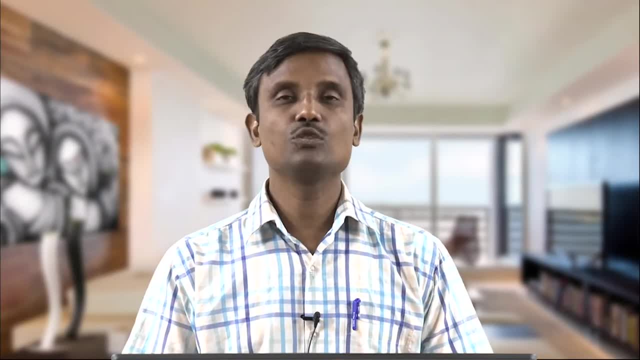 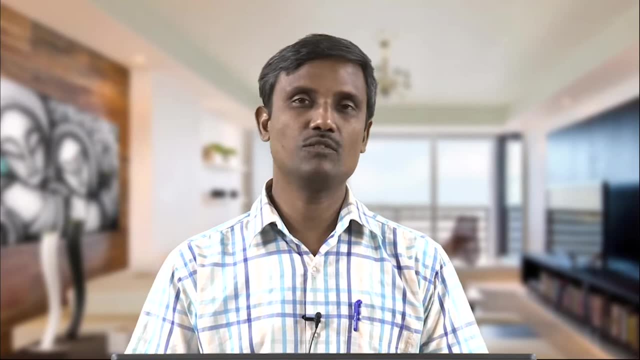 in terms of gamma. you use the gamma detectors. So what should be the choice regarding the detectors? What are the considerations? What are the ideal properties? I what types of detectors are preferred for experimental nuclear astrophysics? Let us try to understand in. 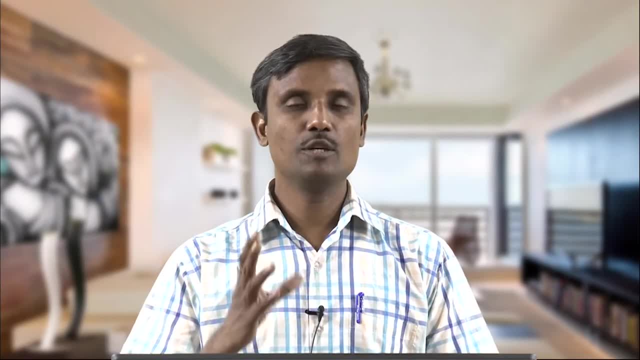 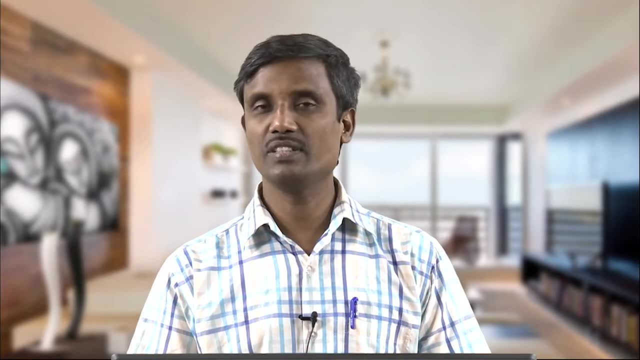 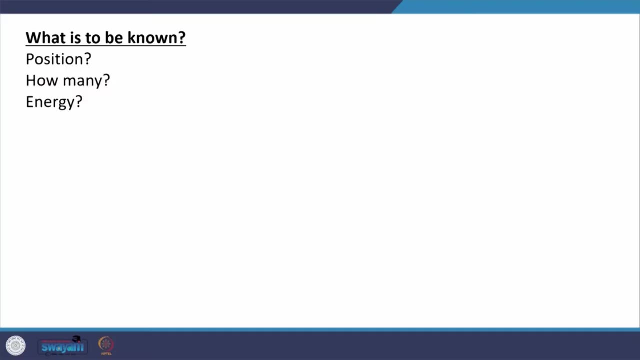 today's lecture cover the basic part of the detectors, which will be useful to understand the response of the detectors when you carry out nuclear reactions relevant for astrophysics. In any nuclear reaction, what should be known? What is the position of the interaction? 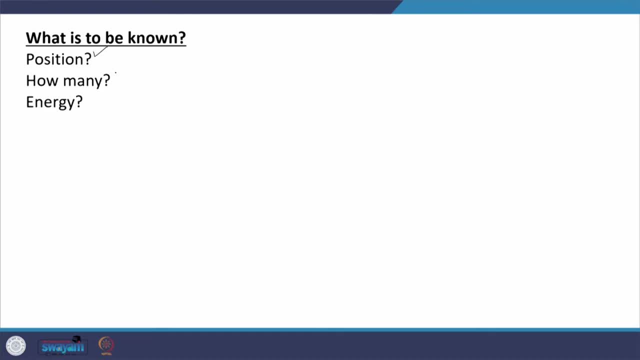 Sometimes you want to see this and many a times. of course, most of the times you want to see the, how many particles are emitted from the nuclear reaction and then, what is the energy of the particle emitted during the nuclear reaction and in how many ways, in how many modes the detector can work? 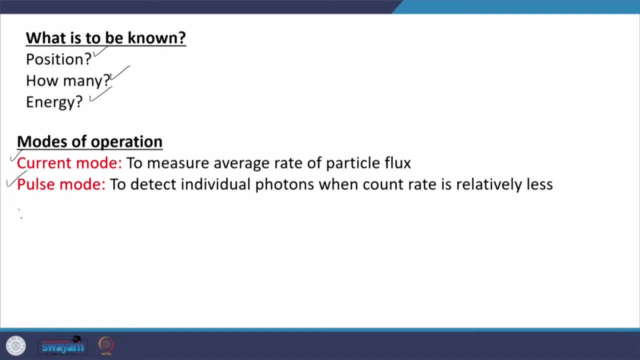 In general we can divide into three types. that is current mode, pulse mode and there is mean square voltage mode. that is not very useful for the our purpose. So in even for nuclear astrophysics, normally we prefer pulse mode. ok, So in the current mode, normally we try to measure the average rate of particle flux. 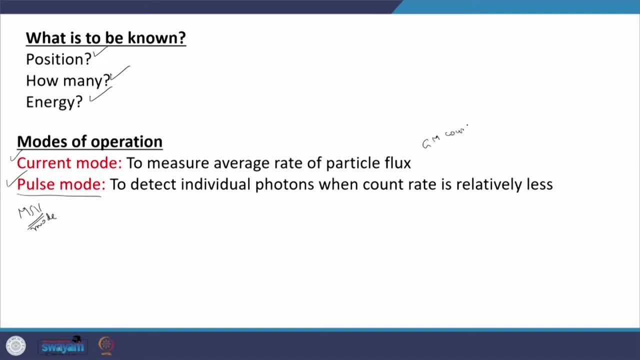 This is used basically. for example, if you go for GM counter or ionization chamber you can use in the current mode to know the average rate of particle flux and when count rate is relatively less and when you detect the individual photons or any other particle and 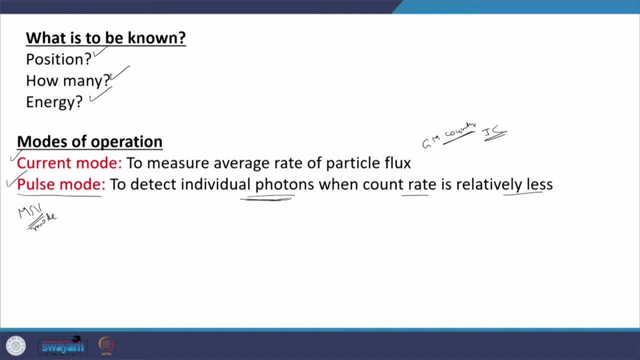 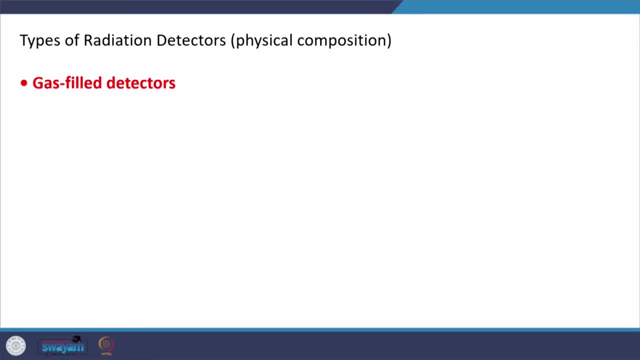 if we want to To measure the energy, then one has to go for the pulse mode. alright, How many types of radiation detectors are available? in terms of physical composition, One can have the gas as the detection medium, one can have the solid, for example semiconductor. 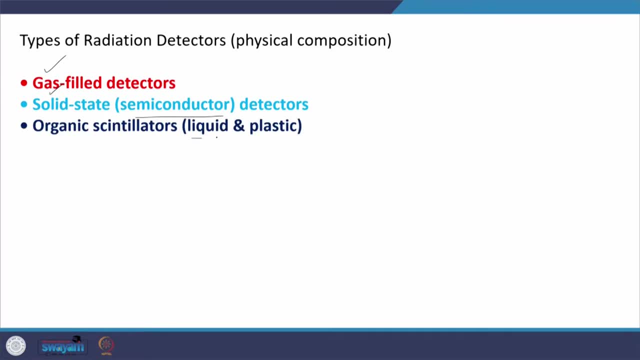 detector, and then organic scintillators, either liquid or in plastic mode, or inorganic scintillators. of course this also comes under the solid state. However, inorganic scintillators are separated from the solid state. Ok, from the solid state, just to differentiate from the semiconductor detectors. Otherwise, 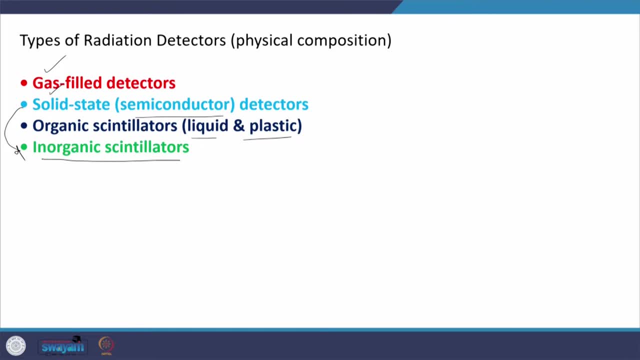 inorganic scintillators. they are also solid materials. The detection medium is solid material And mainly we prefer scintillators for the detection of gamma rays- and many times for the neutron as well, which operate with a photosensor, because material which scintillates that is. 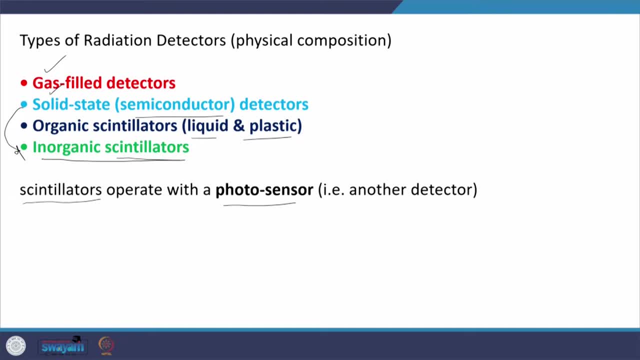 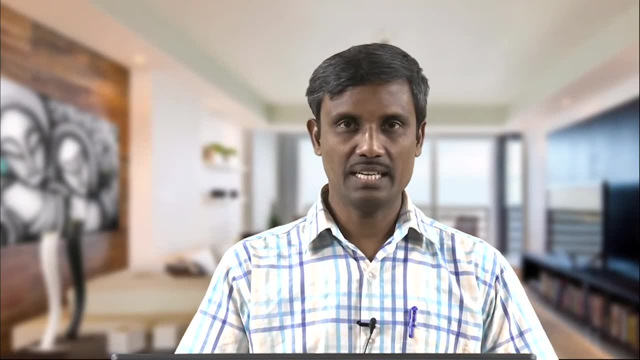 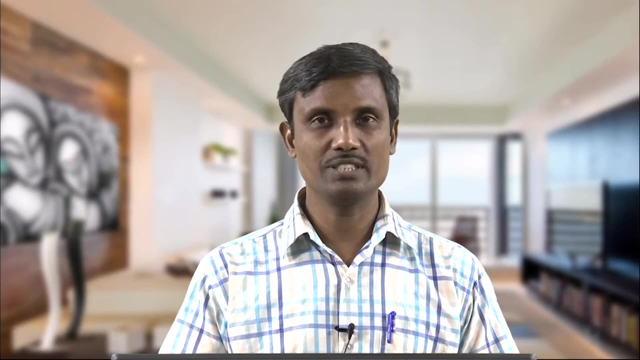 the material which gives photons in visible region, normally, ok, They are called as scintillators, And to detect these scintillations- that means optical photons- one need to use the optical photosensor. ok, One can use the photo multiplayer tube or one. 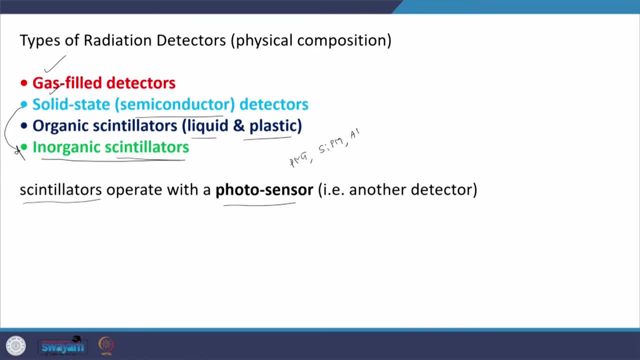 can go for silicon photo multiplier, one can go for avalanche photodiode, one could go for simple photo diode. Ok, So there are different types of photosensors, which itself is a detector of optical photons emitted by scintillation material. all right, 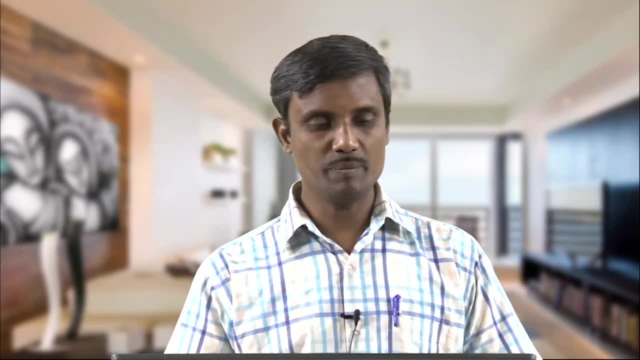 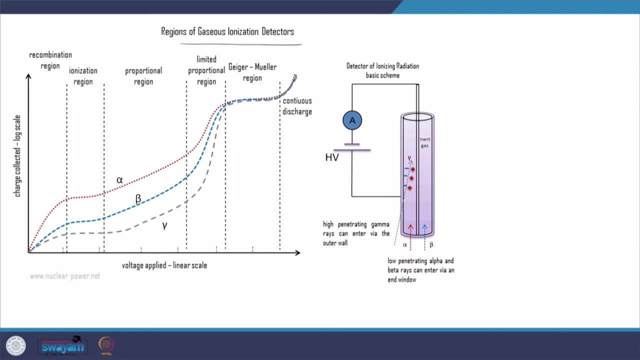 So let me start with the gas detectors. hope you have been taught in your BSc The gas filled ionization detectors which works in different regions, like recombination ionization, proportional, limited proportional and Geiger-Muller counter Geiger-Muller region. 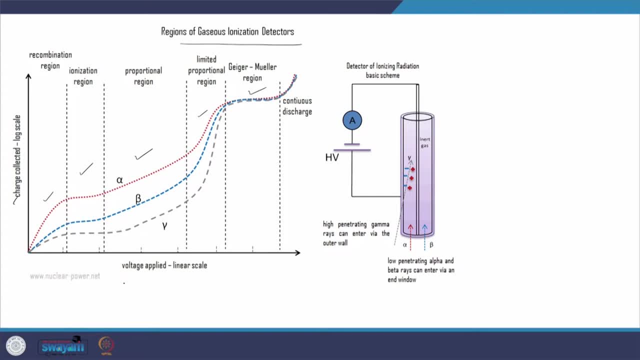 And if you plot this: charged, collected, collected charge and the applied voltage, this is in linear scale and this is in log scale, Initially, when, because of the ionization and excitation, charge carriers are created. charge carriers are created Under the influence of electric field, which is generated because of the applied voltage. 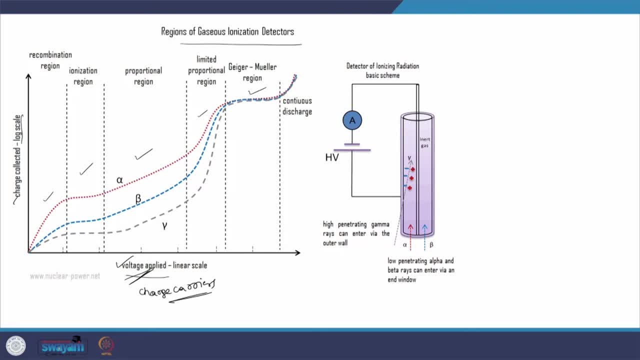 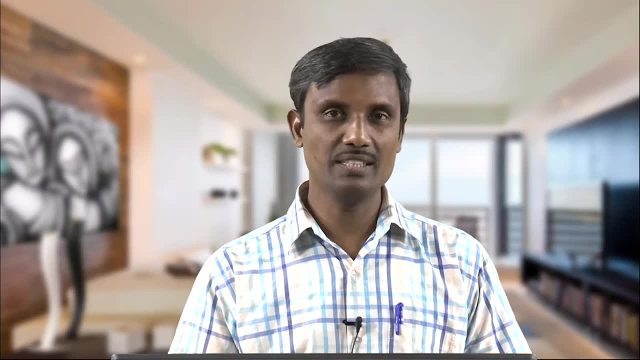 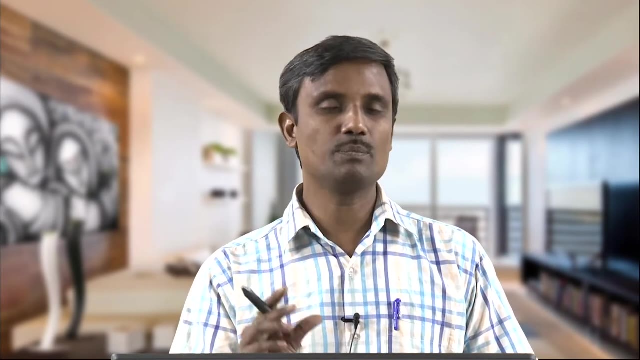 the applied voltage causes the electric field to exist in the active volume of the detector. In the presence of electric field, the charge carriers will undergo drift, And when electric field is quite small, it is not, which is not sufficient for the charge carriers. 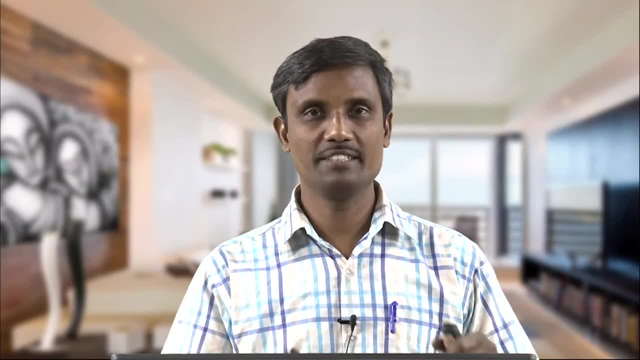 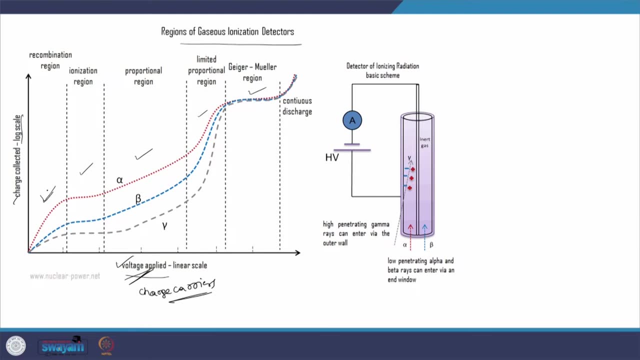 If the charge carriers get collected at respective electrodes, then they will recombine. So that is what I am saying: in the first region- recombination region- Charge carriers will be formed and they will be recombined. Of course, the probability of recombination will decrease as electric field increases. 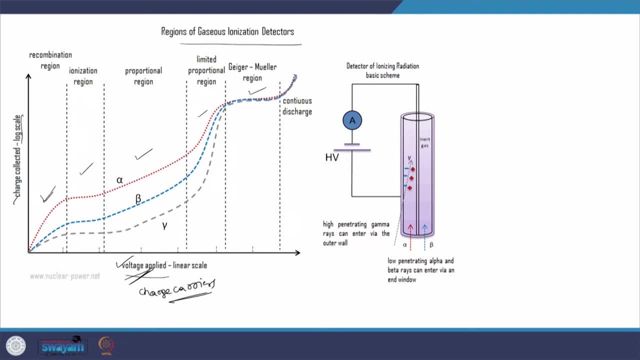 So slowly it reaches to a saturation kind of thing. And once the recombination becomes almost 0, then the region up to which the charge electrode remains same is called as recombination. So the recombination is called as ionization region. 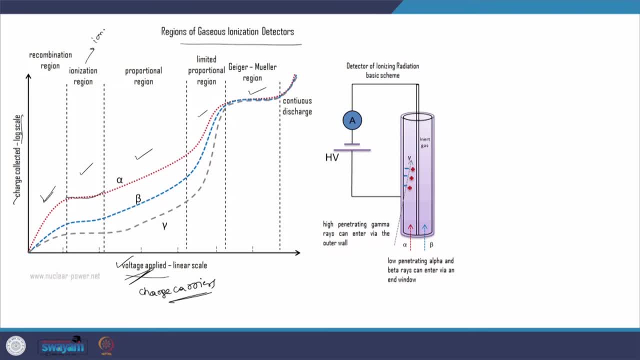 And a detector working in this region can be called as ionization chamber, And sometimes, as part of advanced instrumentation in nuclear astrophysics, researchers are using segmented ionization chambers. So when you come across ionization chamber, it means a detector which works in the ionization. 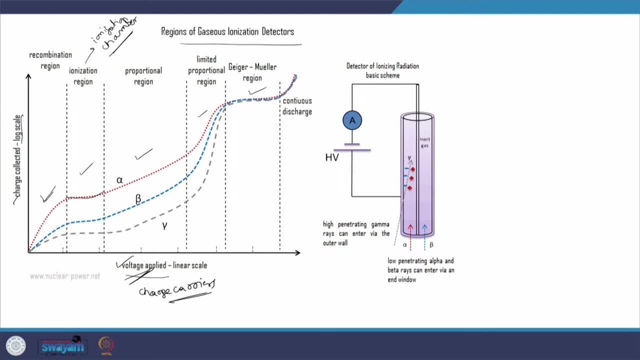 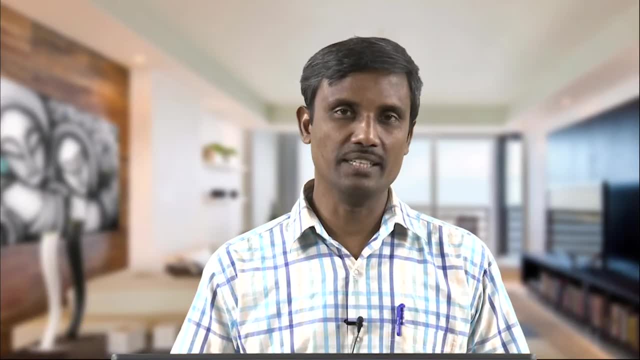 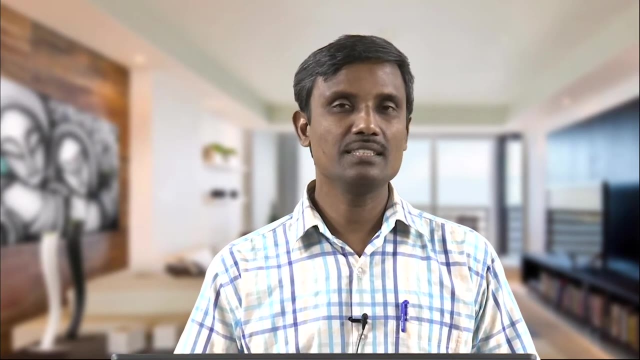 region Where the charge collected is saturated, it is a constant with respect to the voltage. But will it be same Always? no. After certain electric field, there is a process which starts developing within the active volume, That is the multiplication which reach to the proportional region. 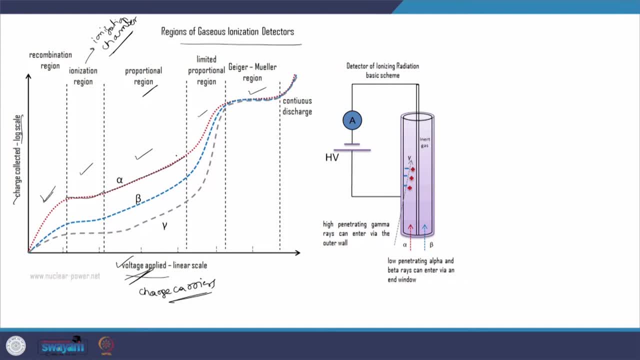 So this linear linearity in the increase of charge collected corresponds to the proportional region, And once this linearity gets disturbed, So this linearity gets disturbed, You are entering into the limited proportional region And after that there is no relation between the incident energy and the number of charge. 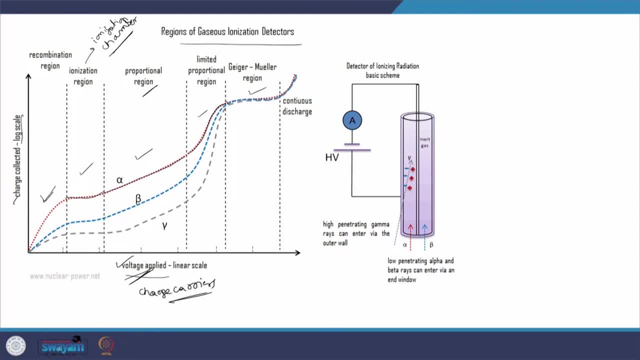 carriers collected because of the avalanche which gives rise to Geiger Muller region, And how this characteristics of gas field detectors looks like for alpha, for beta, for gamma, you can see in this diagram. So this is a schematic of the ionization detector. 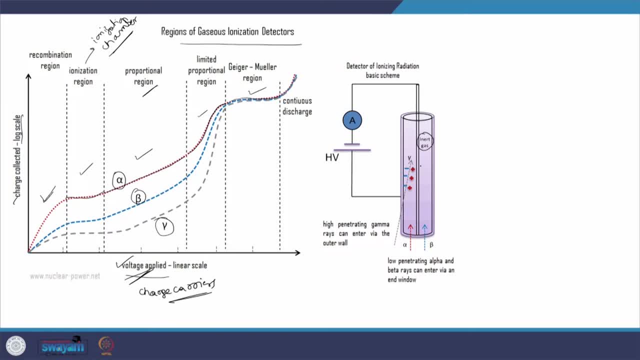 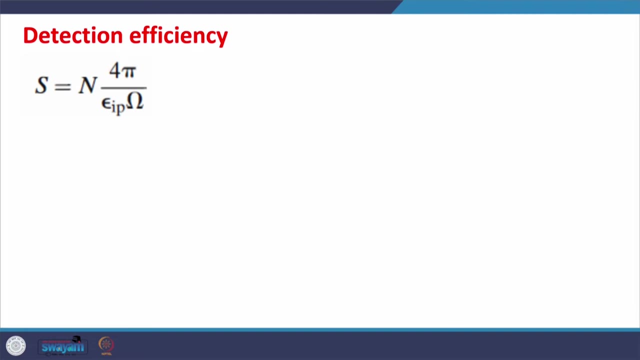 So there is an inert gas we take normally. So any radiation when deposits energy, so they will cause ionization and excitation And under the influence of electric field the collection of charge carriers takes place. How to find out the efficiency of a detector? 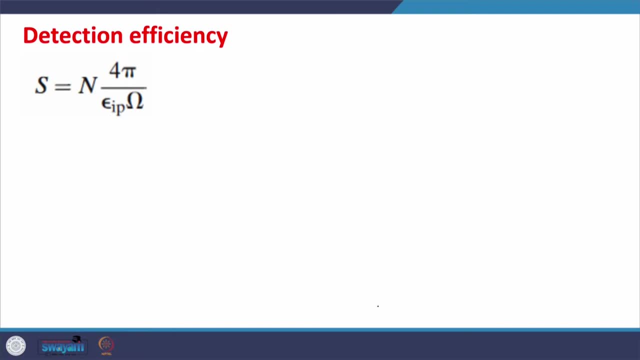 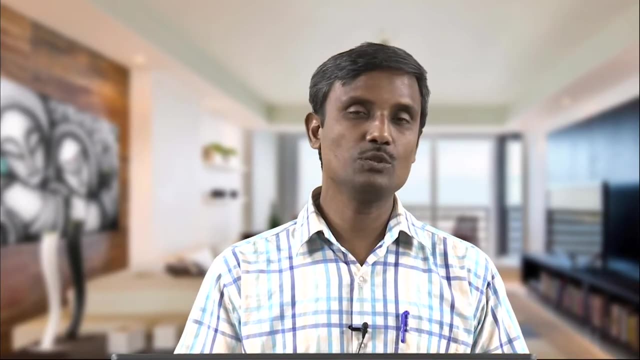 Of course, when we use any detector in the nuclear reaction we prefer to use the detector of high efficiency. So let us see the basics of detection efficiency And once we know efficiency, many a times you can find out the activity of the radioactive source also. 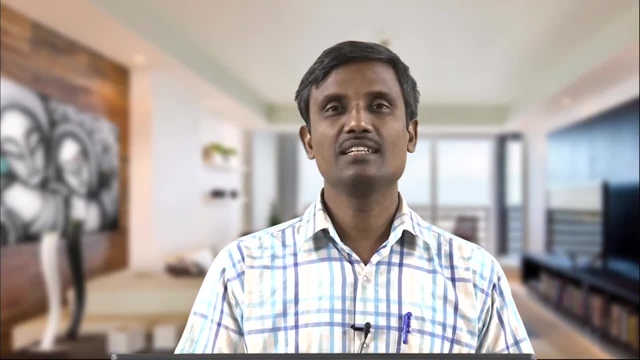 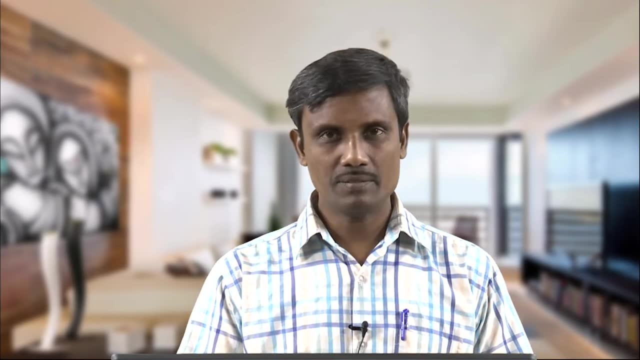 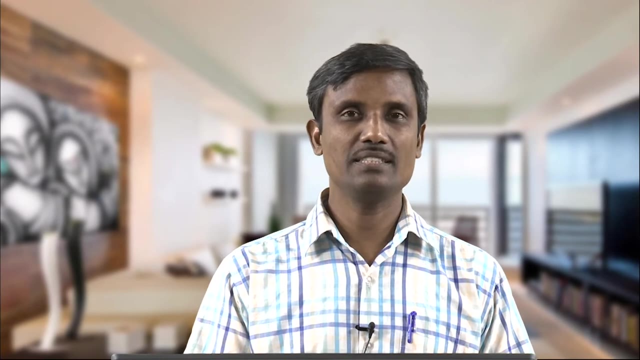 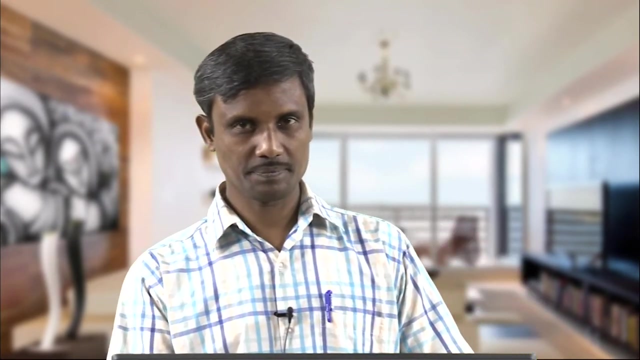 Do you remember, in the previous lecture I have discussed decay schemes of several radioactive sources- cesium, cobalt, sodium, right- and I am confirming my discussion to the gamma rays. in this particular case, when the source emits gamma rays in different directions, What is the number of gamma rays per unit time? 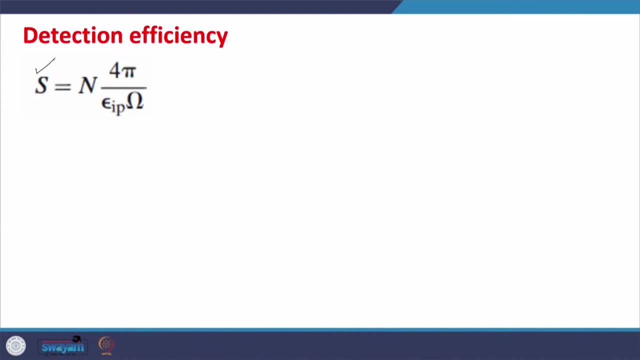 What is activity? Here? I am representing using the symbol S. So S is basically number of particles emitted per unit time, alright, And N is the count Counts under peak of the spectrum. Pi is a constant, 4 is a constant, and this is the intrinsic photopeak efficiency. 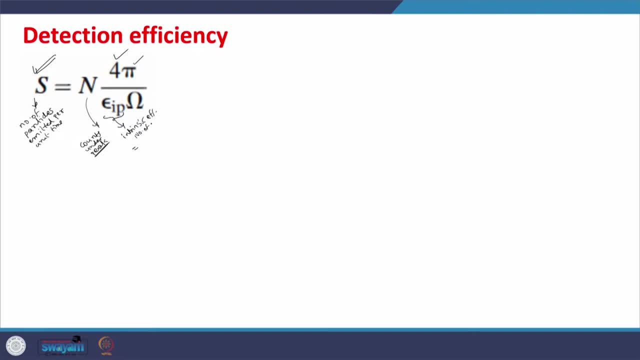 That means number of particles detected under peak divided by Number of particles falling on the surface. falling on detector surface. Omega is the solid angle subtended by the detector at the source. solid angle subtended by detector at source. Okay, Which is given by. 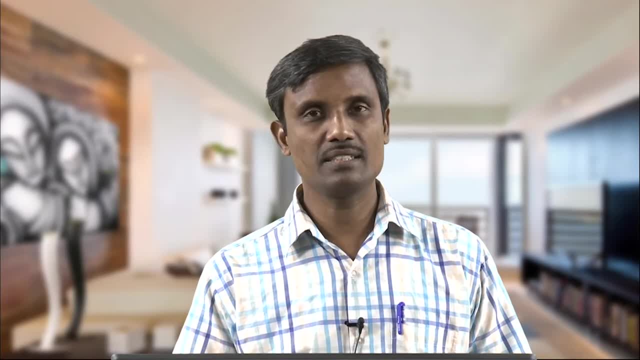 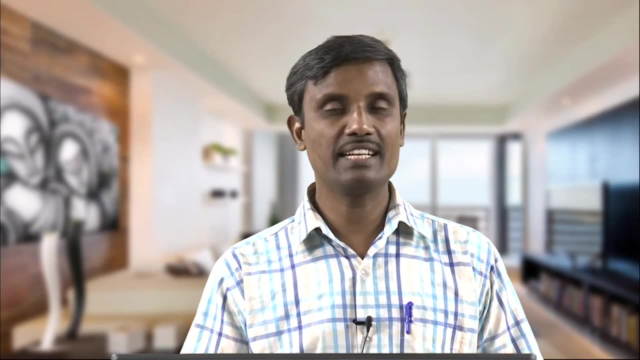 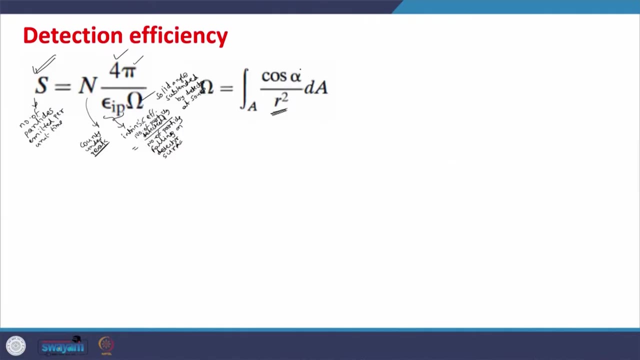 What is the solid angle? solid angle subtended by the detector at the detector surface. Of course it depends on the distance between the source and detector, So you have to integrate the detector surface area over the distance between the source and detector, and where alpha is the angle between the normal of the area element and 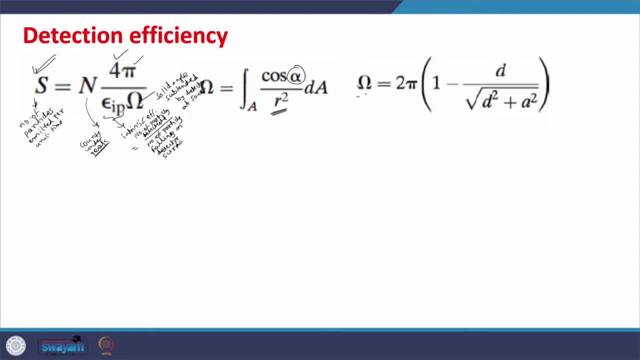 the source point. Okay, So here for a common case of source, and if you have a right circular cylinder, this is for right circular cylinder. We can write down the solid angle as 2pi into 1 minus d by d square root of d square plus. 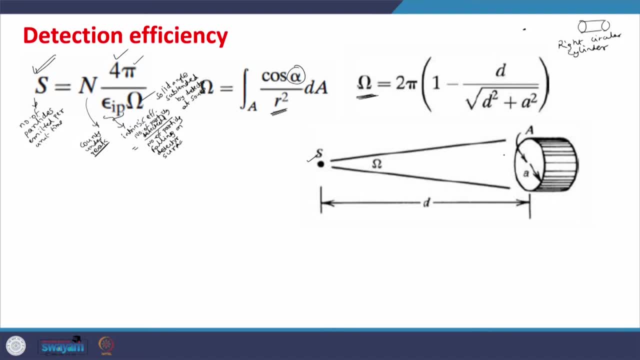 a square. Okay, And here you have the source. You have the right circular cylinder. The distance between source and detector is d. Omega is the solid angle subtended by the detector at the source and small a is the radius of the detector front surface. a is 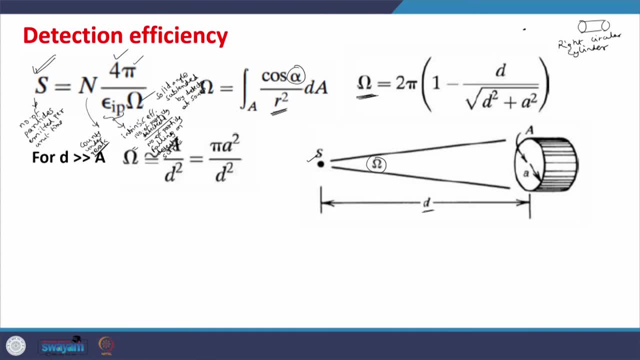 the area of the detector front surface. If this distance is much greater than the area of the detector front surface, then this solid angle can be approximated as area divided by d square, and this area is nothing but pi into square of the radius of the detector front surface. 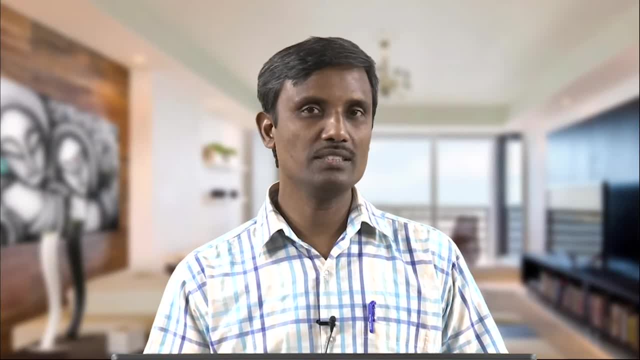 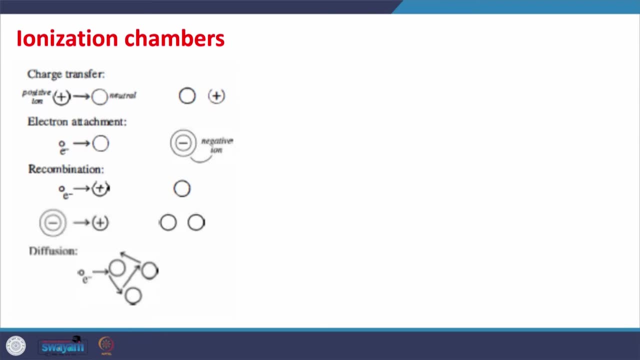 Now let us see more about the ionization channel. Okay, Okay, When charge carriers are created, how many types of reactions can happen? See in the gas medium. when positive ion is created, it can always transfer its charge to some neutral atom or molecule and charge exchange can take place. sorry, charge transfer. 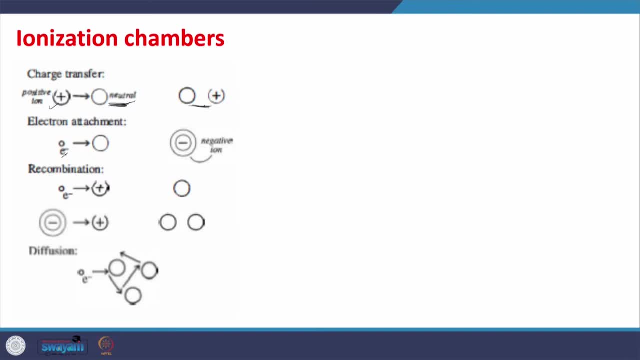 can take place And sometimes electron attachment can happen. So this electron and positive ion, they have been created. They have been created because of the ionization and excitation within the gas medium by the incident charged particle Alright. So electron can undergo attachment with the atom or molecule and positive ion also can. 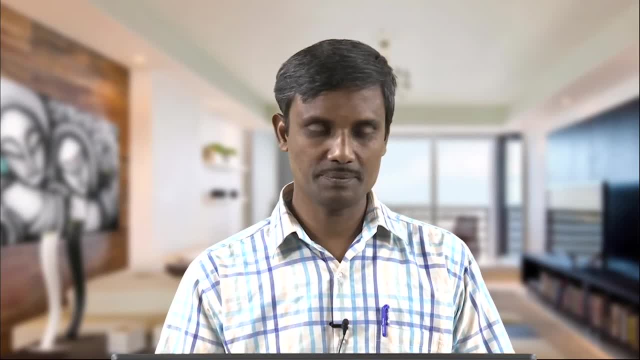 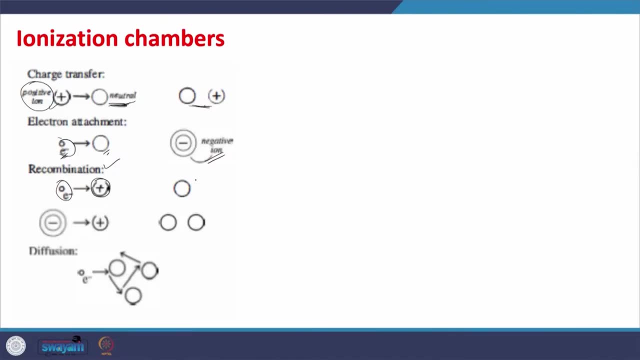 undergo attachment with the atom or molecule of the gas. So then you have negative ion in this case and the recombination also can happen. That is the first region. if the probability is more So, electron and positive ion can give rise to some neutral. 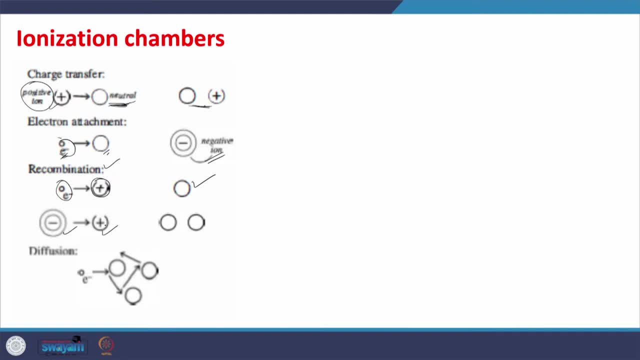 And sometimes the negative ion can react with the positive ion, gives rise to two, neutral one, and diffusion also can happen when atoms or molecules are considered how the diffusion of electron takes place. So all these processes are possible within the gas medium. How much pressure should be applied? 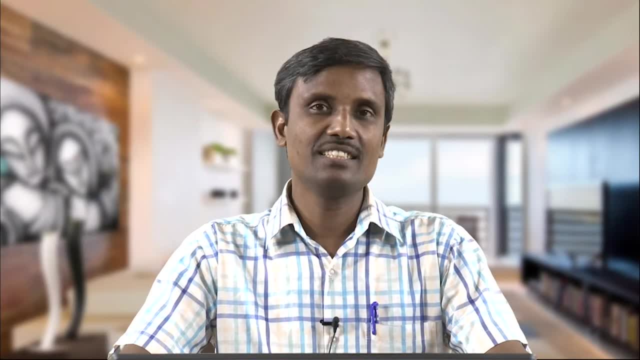 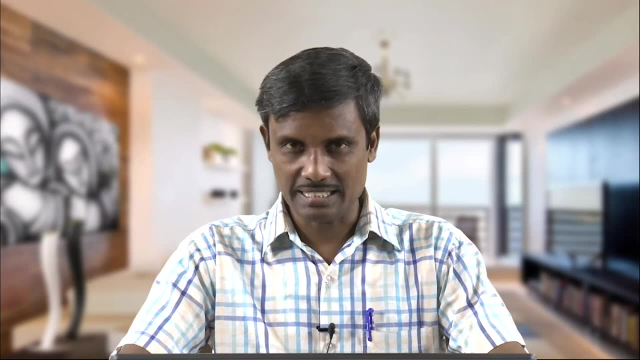 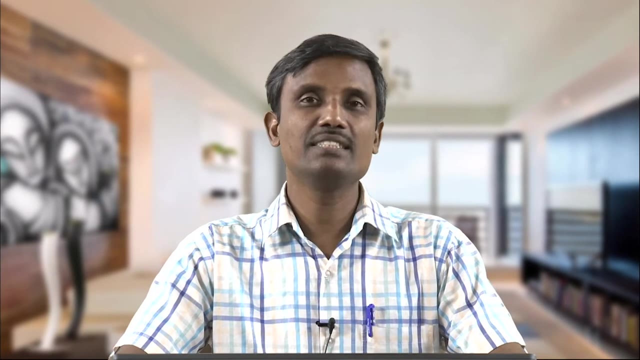 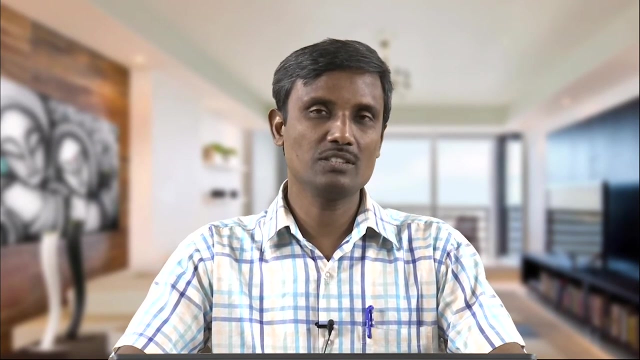 How to choose the pressure of the gas so that it can be used as a proper detector. Okay, So one of the important consideration is the drift velocity of the charge carriers should be almost constant when there is a change in the electric field. Even though you maintain the voltage constant, that means electric field is a constant small. 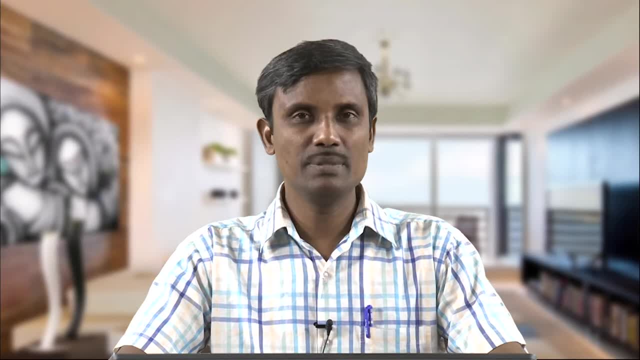 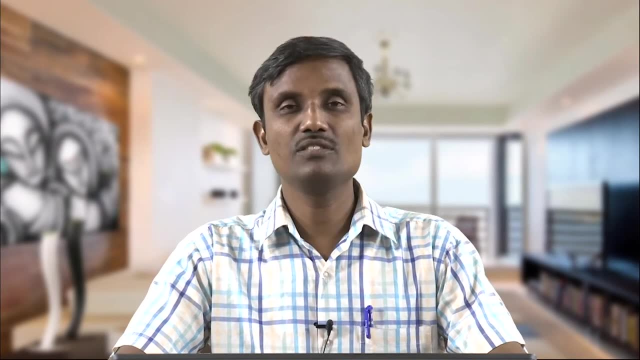 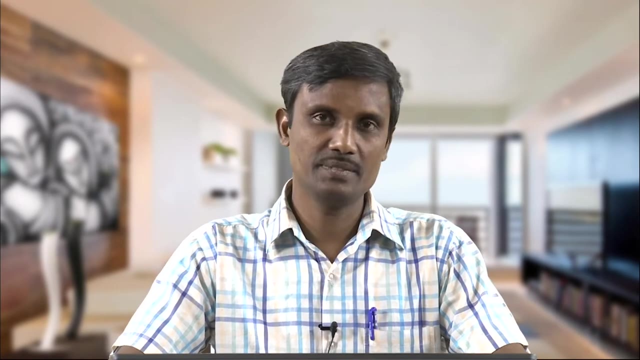 change in electric field sometimes can cause big change in drift velocity. What will happen? Change in the drift velocities can gives rise to two neutral Okay. Change in the drift velocities can gives rise to change in the collection times And change in the collection times can gives rise to change in the pulse height. 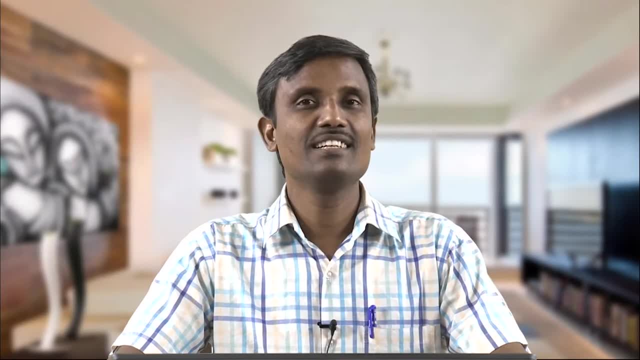 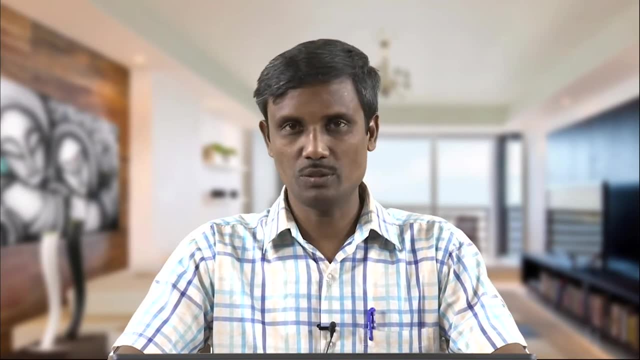 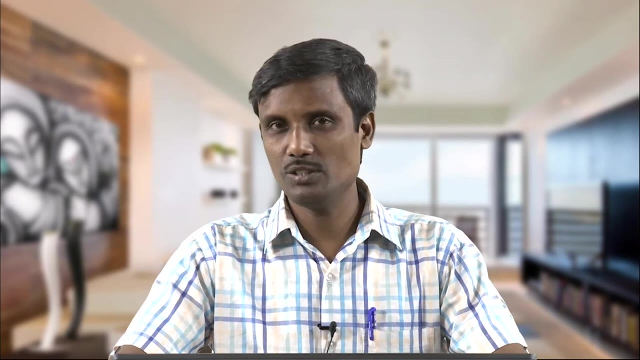 Listen carefully and understand. And change in the pulse height can gives rise to huge error in the energy measurement. So that is how it will hamper our purpose of the nuclear reaction. So it is important to choose proper electric field when gas medium is used in the detector. 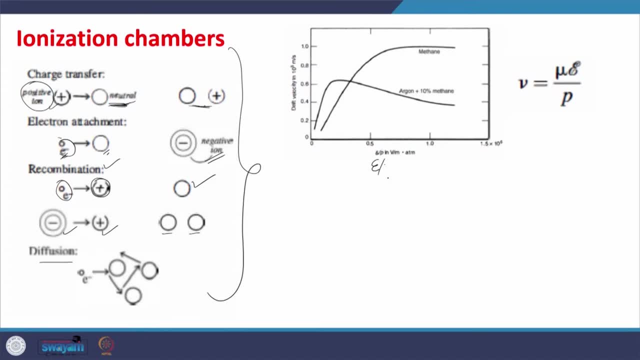 Okay, So the criteria is following: Electric field divided by pressure in voltage meter. atmosphere May be this is not visible, So I am writing for you clearly. Electric field divided by pressure on x axis, Drift velocity in 10 to the power of 5 meters per second. 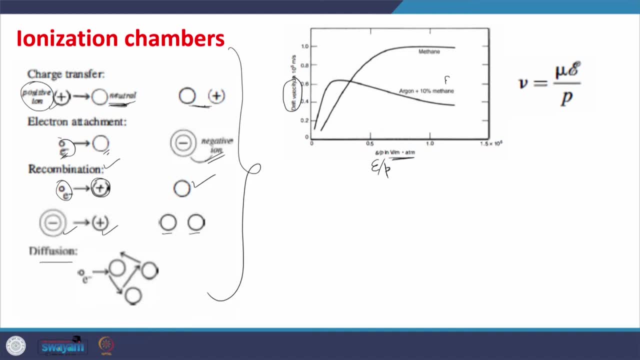 So normally used gas is P10, which is 90 percent argon, 10 percent methane, And normally this is chosen Here. the drift velocity is constant And if methane is used, Of course you can use 0.6 to say 1.2 volt per meters atmospheres. 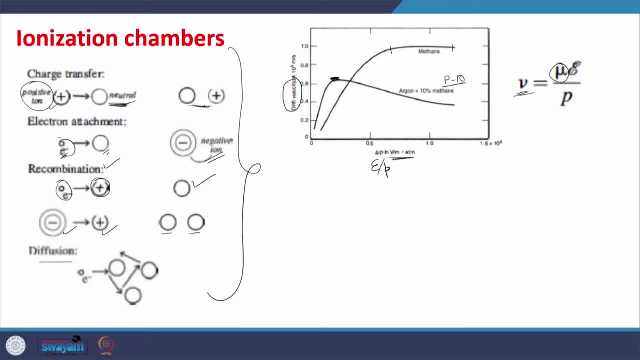 And the drift velocity is given by the mobility of the charge carrier, electric field and the pressure of the gas. Alright, And just for your information, this table gives you values of energy dissipation per ion pair which we use where we use the symbol W. 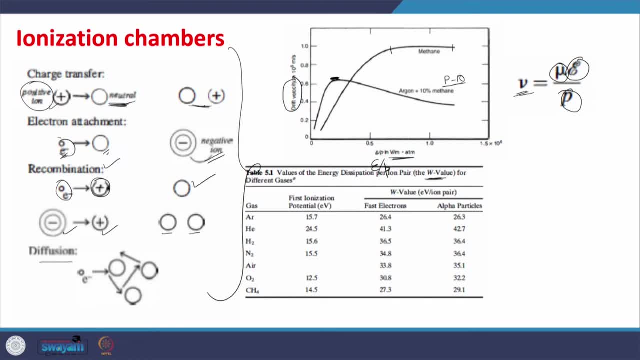 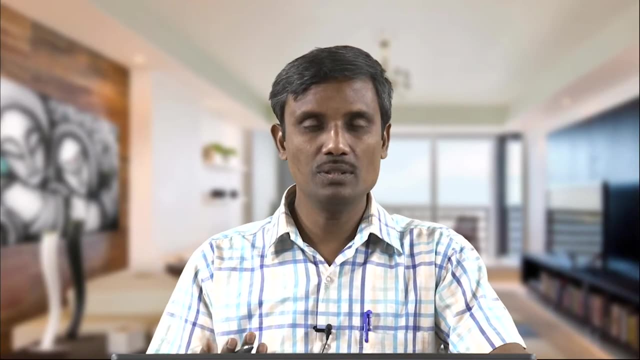 Energy required to produce Energy. required to produce Energy required to produce one electron ion pair in case of gas, or one electron hole pair in case of semiconductor or scintillator material That is called as W value: More W value, less. number of charge carriers for a fixed incident energy. 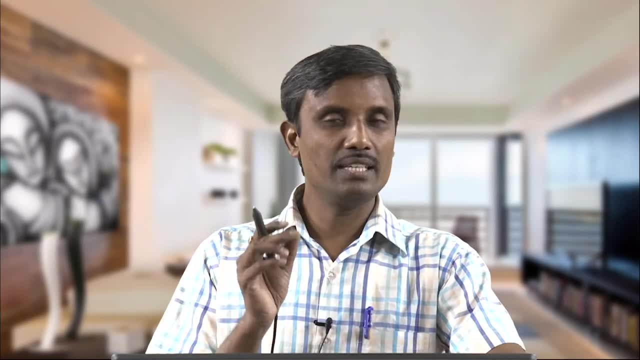 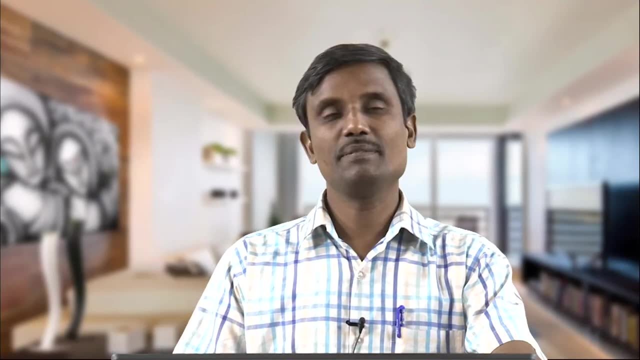 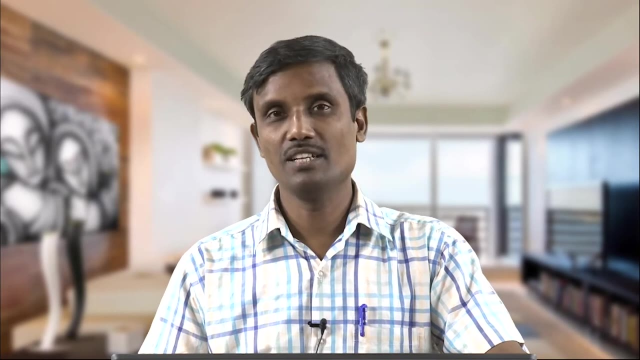 And for a fixed incident: energy: less W value. lesser the value of W, larger will be the number of carriers. So that is where Semiconductor detectors and inorganic scintillator Semiconductor detectors are preferred over ionization chambers for the detection of. 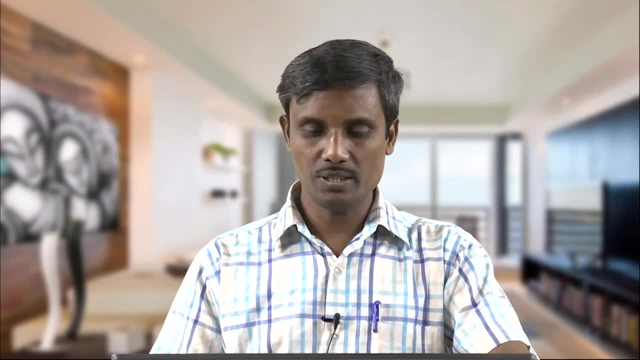 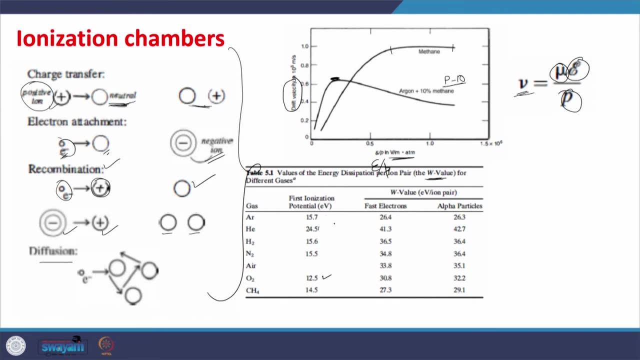 charged particles. Alright, So you can see. the first ionization potential is ranging from, say, 12.5 to 24.5 electron volt And the W value for fast electron it ranges from, say, 27 to 41. So this is the W value. 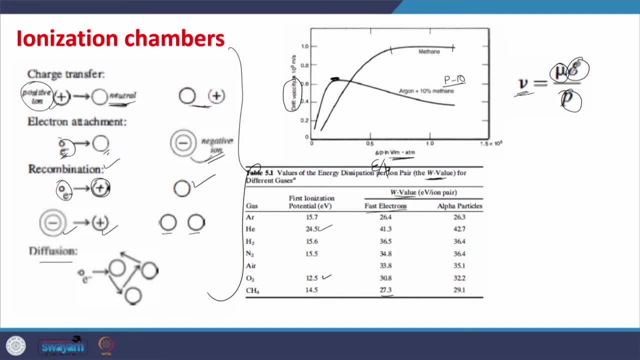 So this is the W value. So this is the W value. And for alpha particles, this is of our interest. And for alpha particles, this is of our interest, Ranges from 26 to 42.7 electron volt per ion pair. 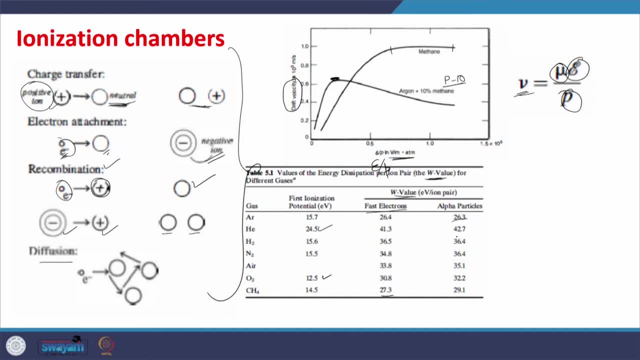 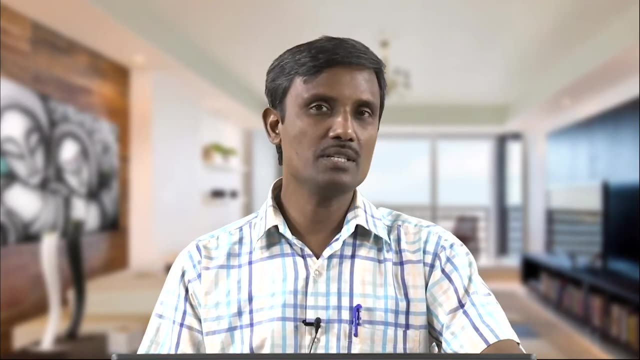 Ranges from 26 to 42.7 electron volt per ion pair. So if you know the W value you can find out the number of charge carriers produced for the fixed incident energy And that gives rise to that gives. that helps us in getting the information of pulse height. 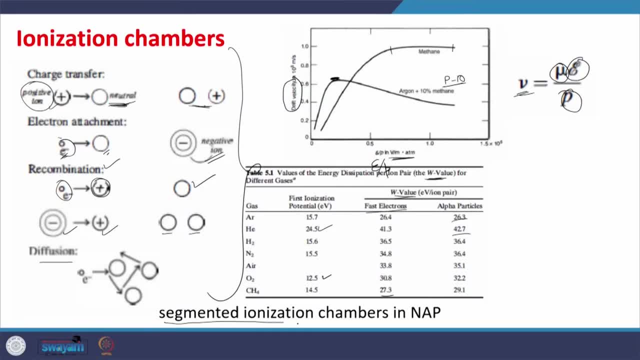 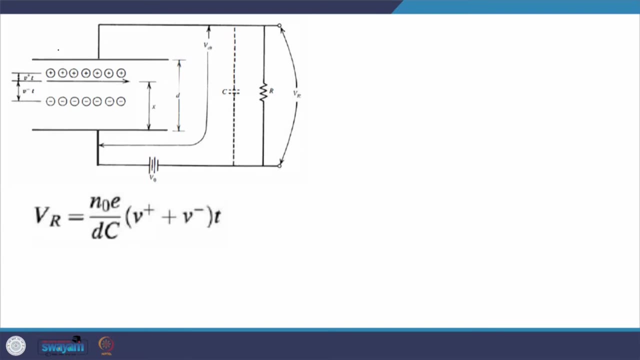 Ok, And as I said, in nuclear astrophysics, as part of advanced instrumentation, people are using segmented ionization And in this slide I have discussed the salient features of basic ionization chamber. Alright, Let me discuss the simplest design of the ionization chamber. 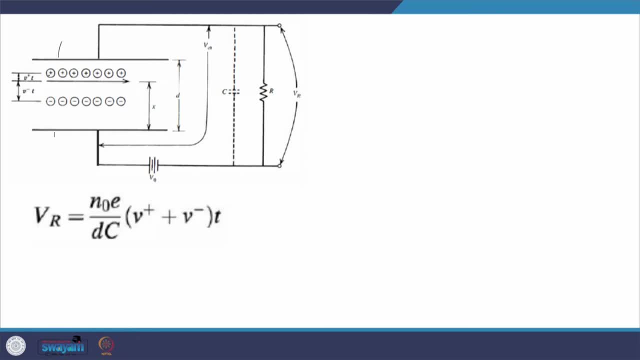 Two electrode parallel plate ionization chamber where this arrow mark ok. This arrow mark denotes the travel of charged particle within the gas and, just for the sake of convenience, These positive and negative charge carriers, they are represented on both sides and they are collected at the respective electrodes. 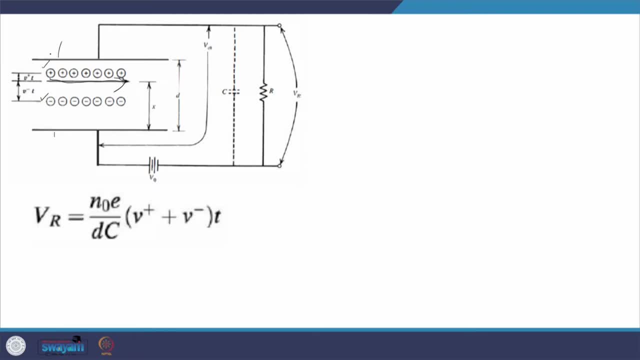 Electrons are collected at the anode and positive ions are collected at the cathode material. Ok, And they have their velocities, with respect I mean- which depends on the electric field within the gas medium And the voltage across the load. resistance is given by number of charge carriers produced. 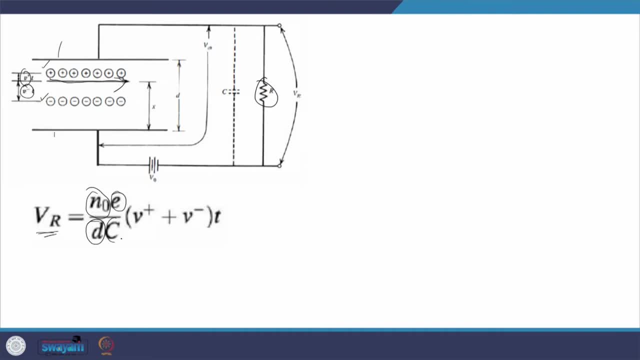 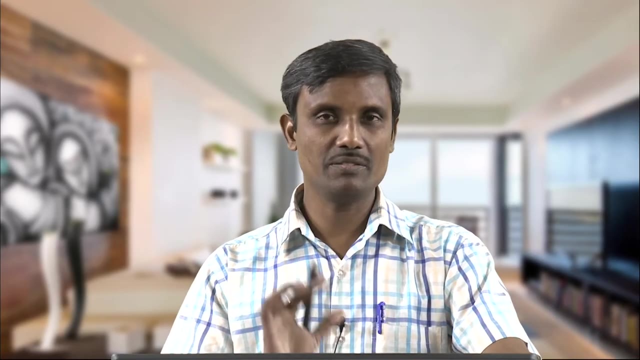 the value of charge. Separation: Separation between the plates. Capacitance, which includes the stray capacitance of the detector and the velocity of the positive ions, velocity of the negative ions, negative particles, that is, electrons. Positive ions are 1000 times heavier than around 1000 times heavier than the electrons. 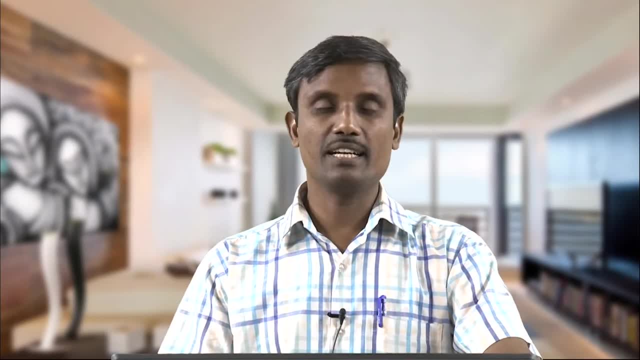 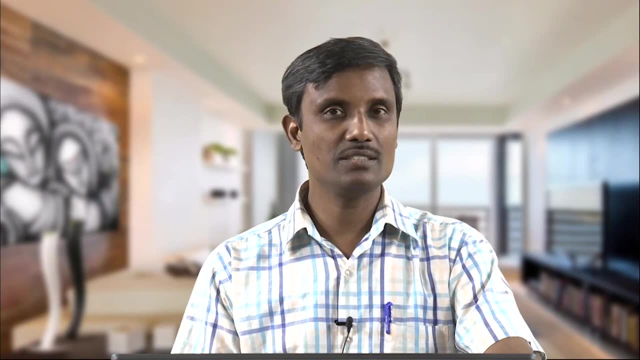 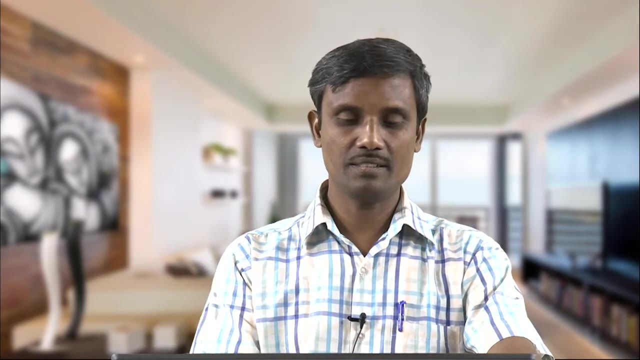 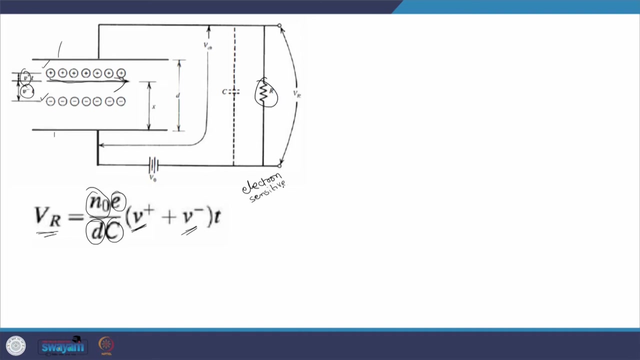 So it will take less time to reach to the electrode. Electrons being lighter particles, it will quickly collected at the anode, So electron will reach the electrode first. That is a reaction. That is a reason Many a times ionization chambers are operated in electron sensitive mode. 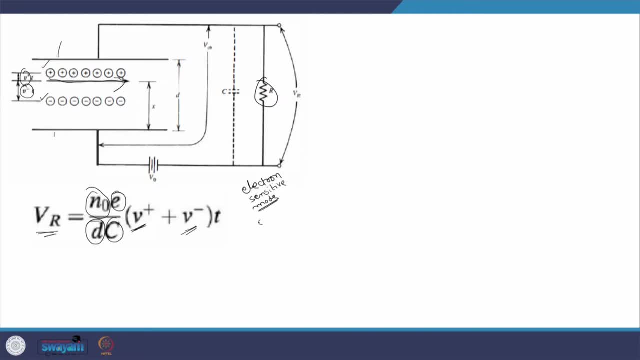 The time constant of the detector circuit is chosen such that it is less than the collection time of positive ions. But I mean tau is less than the T plus. So this is a time. So in this case tau is less than the t plus. 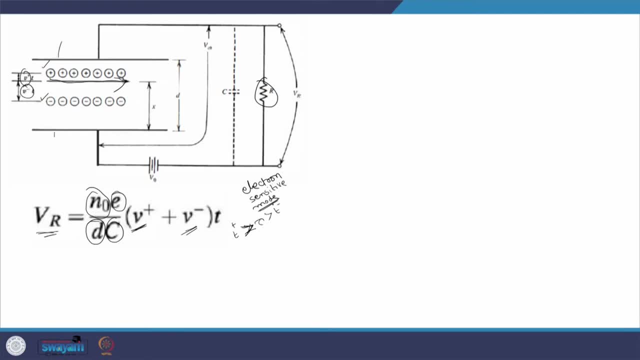 So it is a time constant. Subject: Subject: Subject: Subject: but greater than T minus, that is collection time of the electrons. So it will not consider the motion of the positive ions, otherwise it is difficult to maintain the count rate. 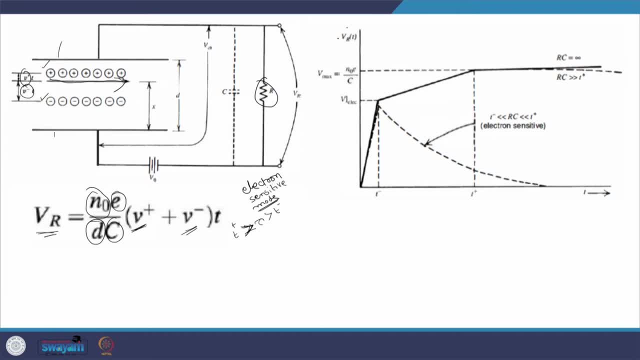 And this is how the time development of voltage pulse across the load resistance takes place. Time on x axis. voltage development across the load resistance on y axis. So up to this: electrons motion, positive ions motion see after electrons are collected. you have so much time for the positive ions to get collected. So that is the reason here I have said T minus. 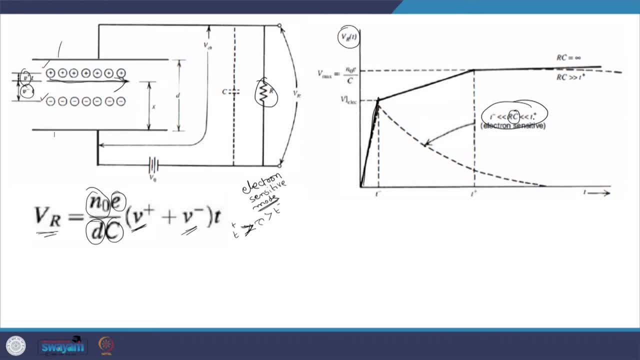 is less than time constant of the detector circuit and which is much less than the T plus electron sensitive mode. ok. And if the time constant is chosen much larger than the T plus, then positive ions collection is also considered alright. So this is how time development. 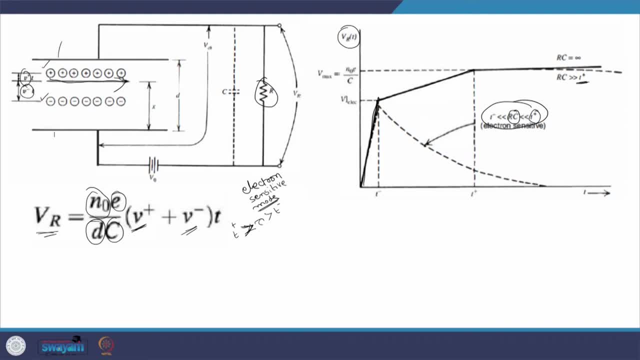 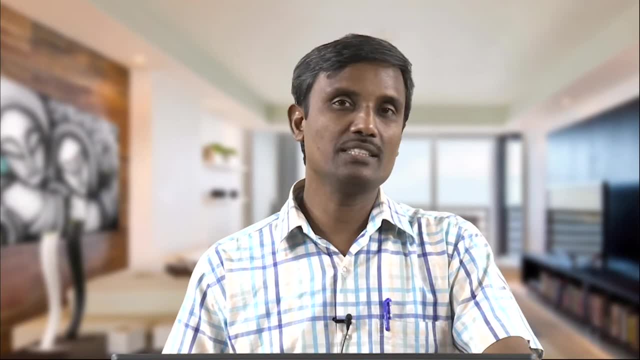 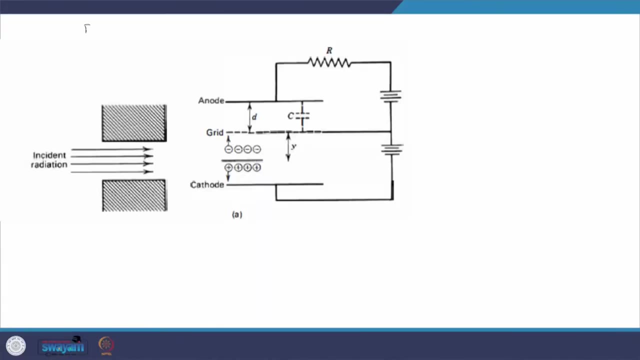 of voltage. pulse can be calculated using conservation of energy. one can derive the formula Now. the problem in parallel plate ionization chamber is the dependence of pulse height on the location of interaction. ok, So this is a very important phenomenon, the dependence of pulse height on location of interaction. 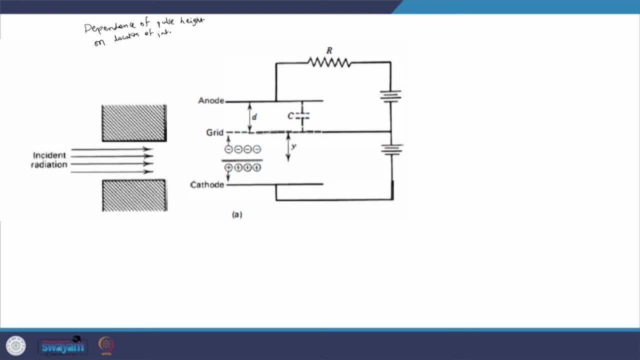 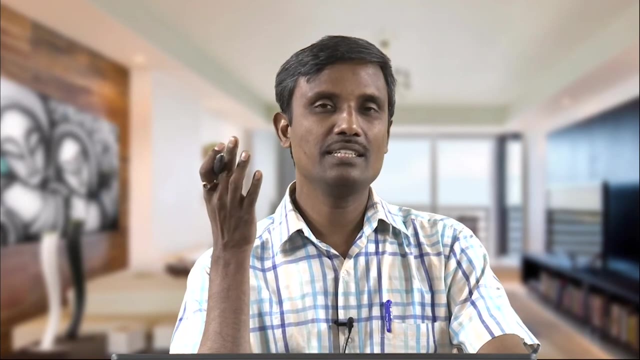 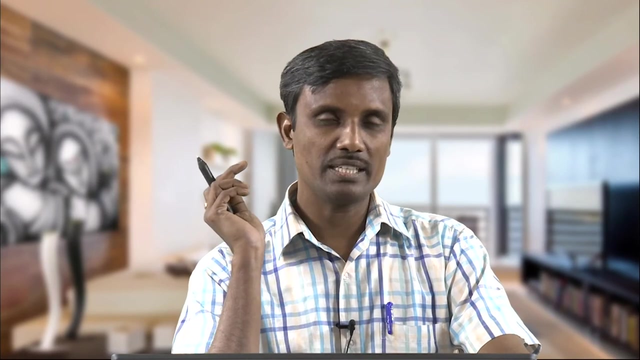 So, depending on the location interaction, if the pulse height changes then the energy measurement will be difficult. For this given energy pulse height is different. two same energies, two particles of same energies, will give two different pulse heights in the case of two parallel plate ionization chamber. But in this particular case we want the energy should. 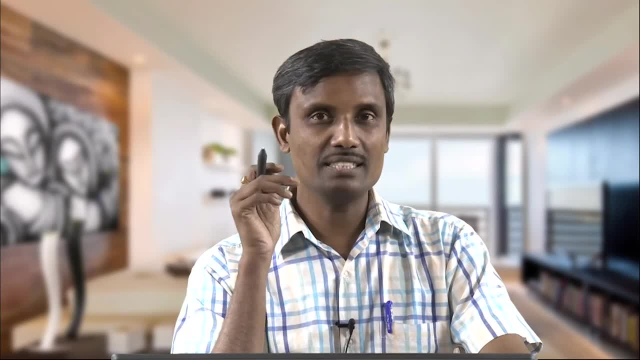 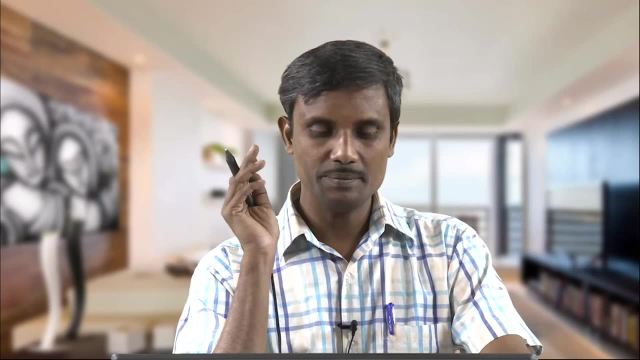 be same as was the original. So in this particular case, we want the energy should be same as was the original. That is the reason grid is introduced between the two plates and the location is confined between the grid and the cathode So that electrons, wherever they are, created once they 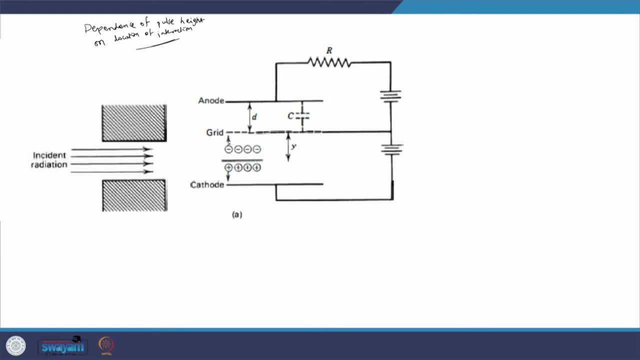 started moving towards the anode, it will not be considered for the pulse formation until it crosses the grid. Here the distance between the anode and grid is taken as d ok. So this diagram help us How to understand, How to understand the pulse formation. Till electron drifts toward the grid, there is no 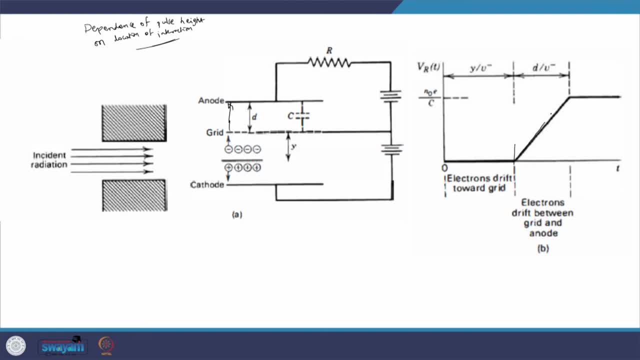 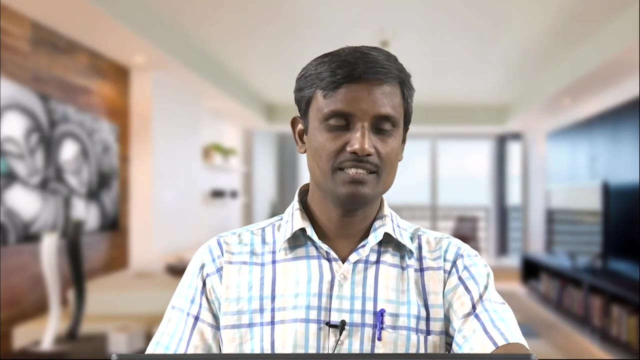 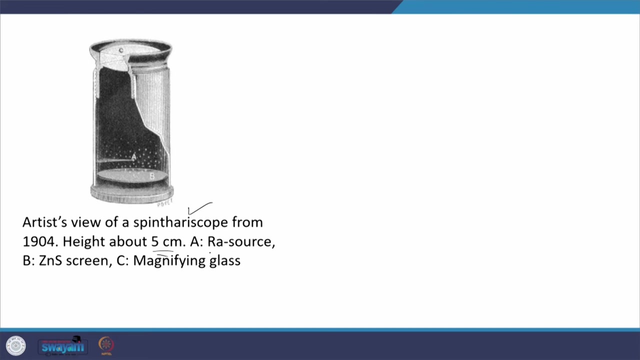 pulse development. and the pulse starts developing after this position. So d minus d by v minus gives you the collection time of the electrons. all right, Then let me discuss the scintillation detectors. the story starts from the spin theriscope, ok, where about 5 centimeter height and radium. 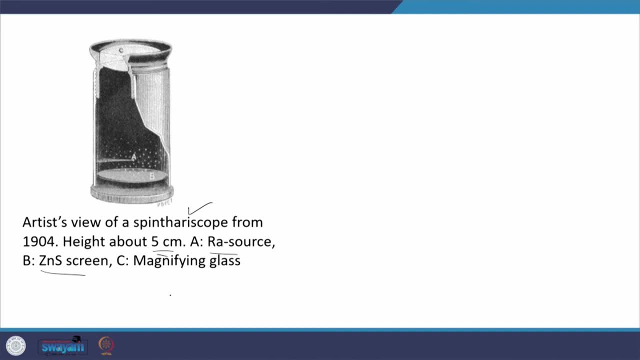 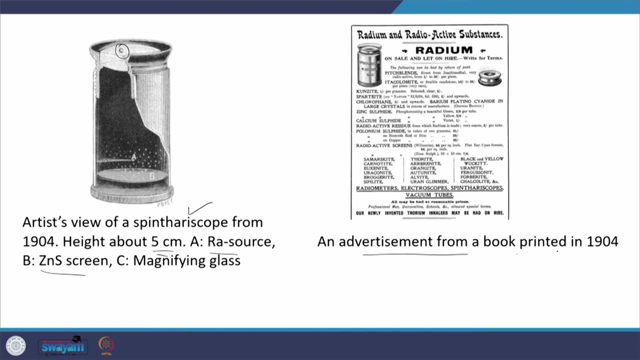 source was used for the alpha particles zinc sulphide screen and here the magnifying lens is used. with naked eye people used to count the scintillations. And one interesting advertisement from a book printed in 1904 you can see here and the details can be found in this paper. 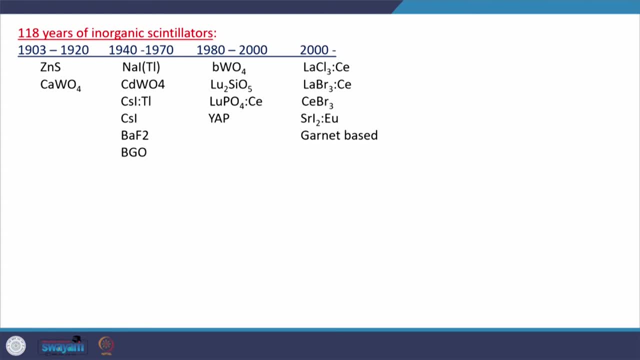 And if you see the evolution of inorganic scintillators, evolution of inorganic scintillators starting from the zinc sulphide, now we have come up a long way. So, starting from time-tested sodium iodide, people are widely using advanced scintillators like lanthanum, halides, cerium. 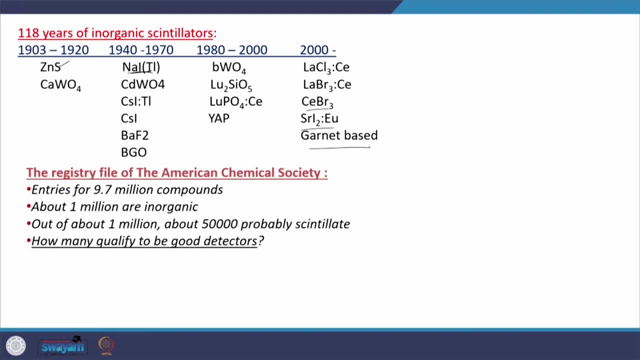 bromide, strontium iodide and garnet based scintillators. If you see some numbers, interestingly, around 10 million compounds are entered in the American chemical society registry and out of them, 1 million compounds are inorganic. out of them, 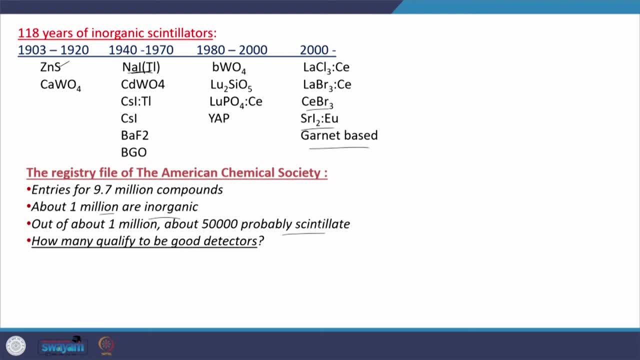 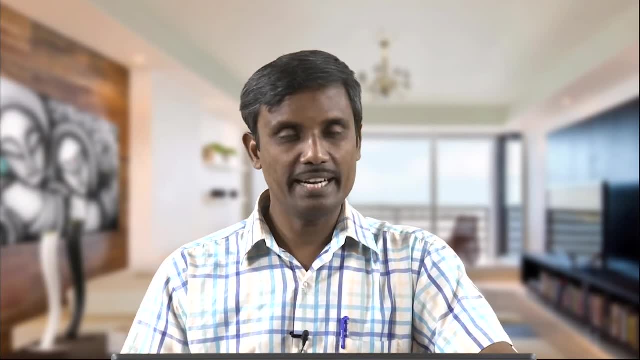 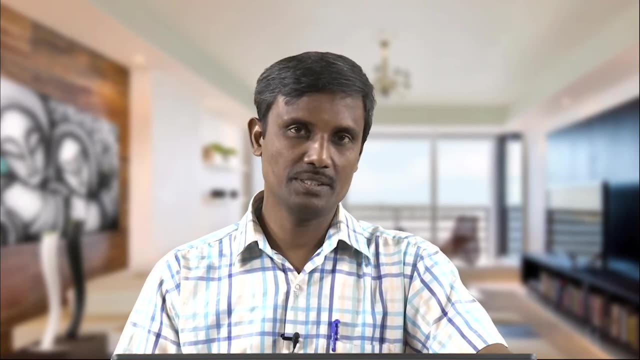 probably 50000 will scintillate, But the question is: out of them, how many will probably scintillate? Ok, So that is a challenge, And what are the properties that we look forward to when we consider any scintillation detector? So, after discussing gas based detectors, 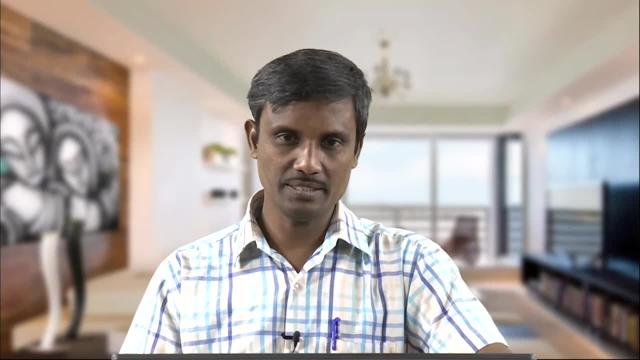 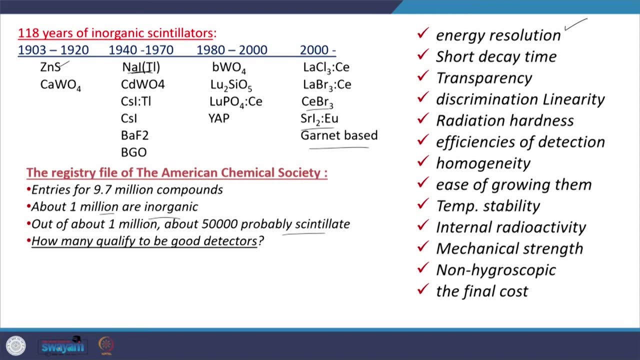 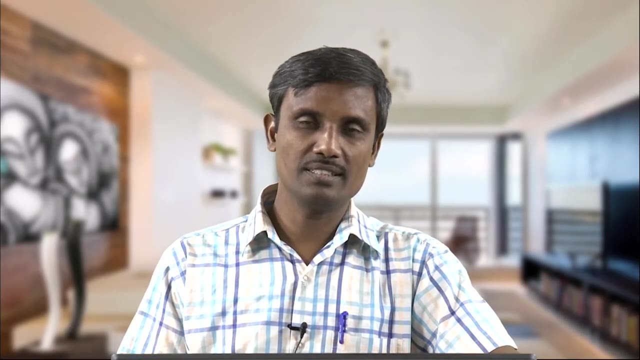 I am discussing now the scintillation detectors. all right, So that is energy resolution, the ability to resolve two energies closely separated from each other. Then, if fast timing is preferred, we of course look forward. the fluorescence phenomenon should happen very quickly, So we should have a short decay time, and then it should be transparent to. 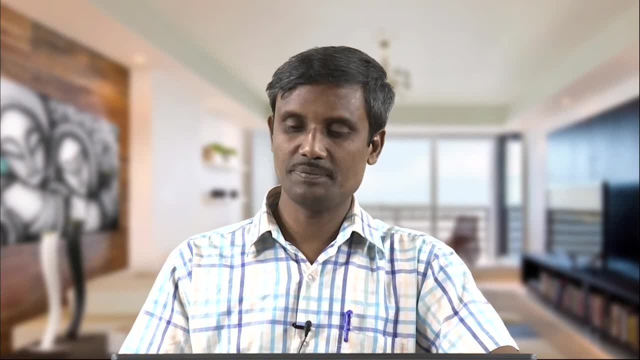 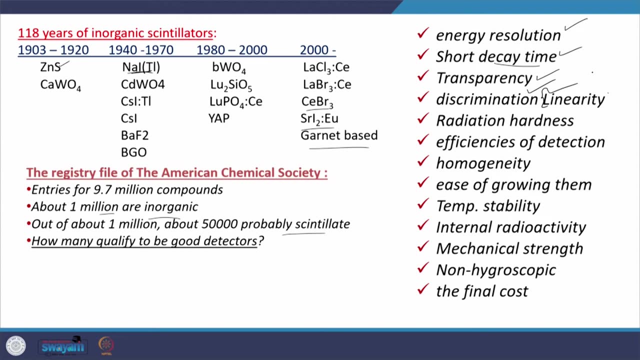 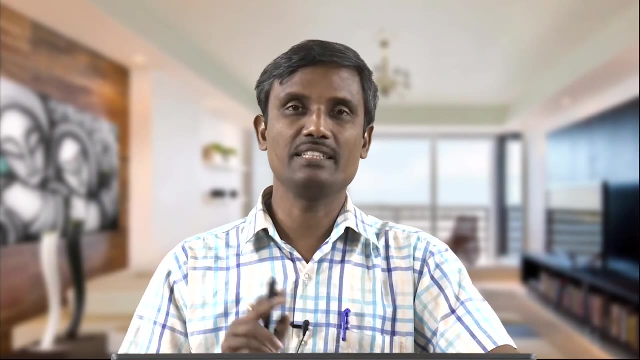 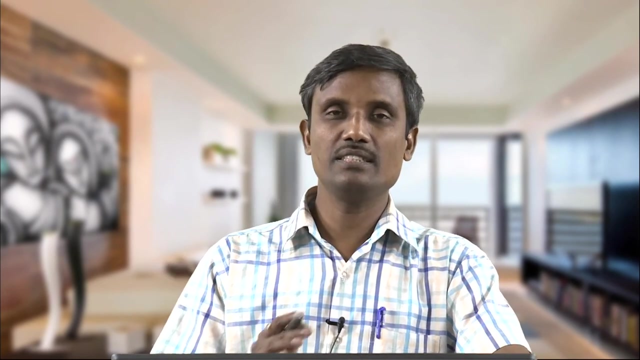 the optical photons generated within the scintillator and discrimination of different types of radiation. and here totally different point, that is linearity of the detector. That means energy. the relation between energy and the pulse height should be linear. So this linearity of the detector can be checked by considering energies, of energies. 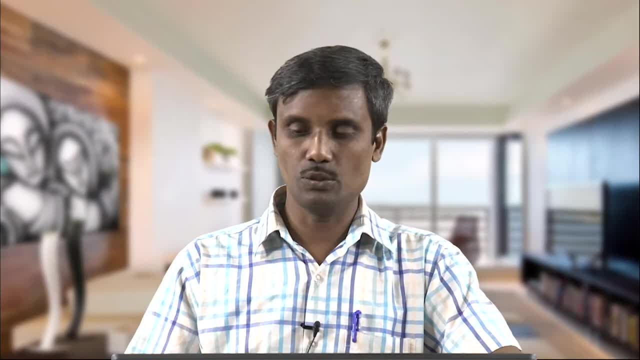 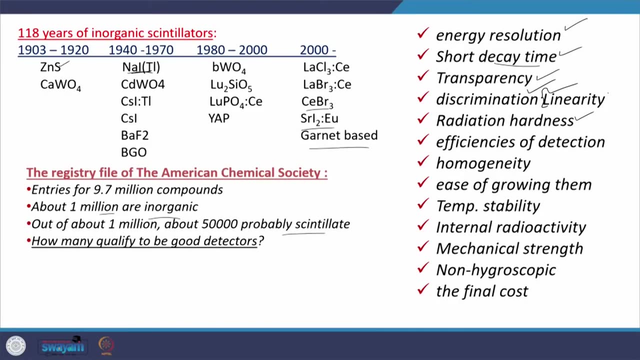 of gamma rays by taking different values, ok, And how hard it is with respect to radiation? Can it sustain the high amount of radiation for long time? And then, what is the ability to detect, which can be categorized into total detection efficiency and full absorption efficiency? 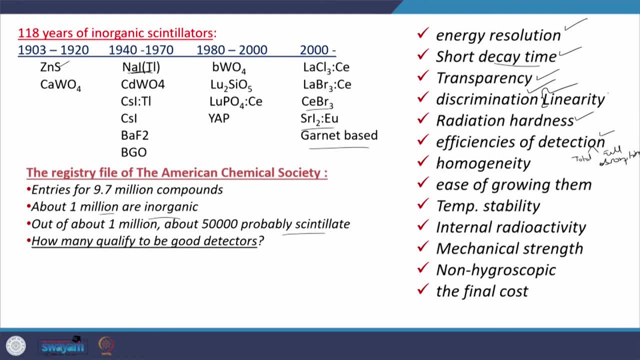 full absorption efficiency. Homogeneity- what is this homogeneity material? If I consider any detector, ok, if gamma rays come through here, through here, through here- see, the PMT is placed here. ok, So if gamma is falling at any point from the side, 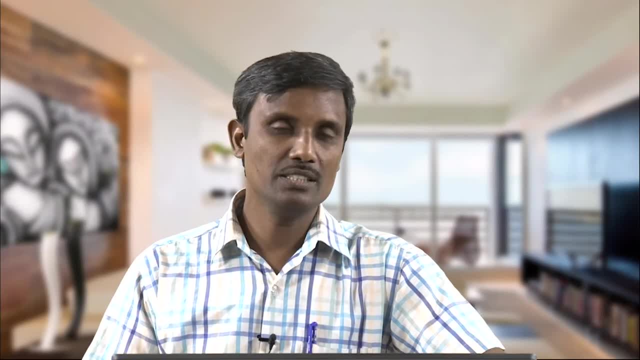 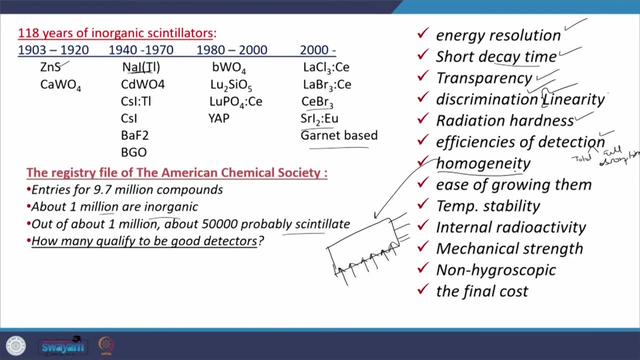 then the performance should not be much different from each other. ok, So normally we call this as lapping also. So homogeneity also has to be checked for the large volume detector And how it is, how easy it is to grow in a large volume detector. So homogeneity also has to be checked for. 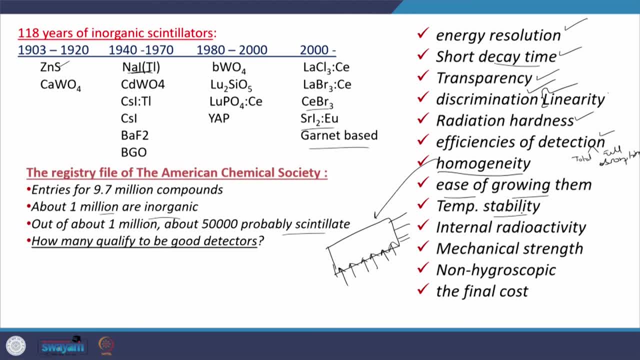 the large volume detector and how it is, how easy it is to grow in a large volume detector. So homogeneity also has to be checked for the large volume detector and how it is, how easy it is to grow in large volume ok, And how stable it is in terms of temperature. Of course, not much relevant for 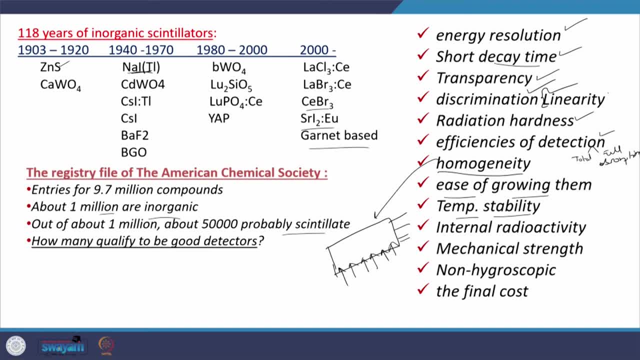 nuclear astrophysics because we are not operating these detectors at the very low temperatures. though it has its own advantages, ok, Detector should not contribute to a radioactivity from own. So detector should not contribute to the radioactivity, otherwise the count rate that we are looking for will be overlapped. 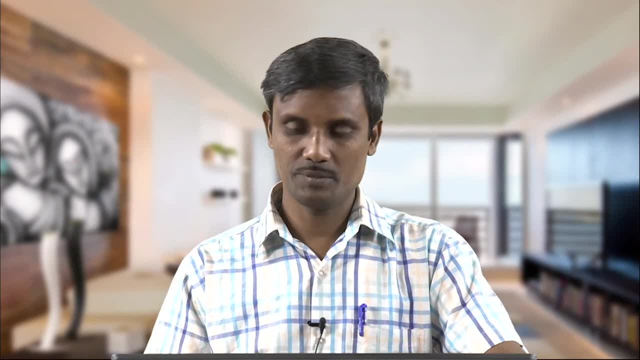 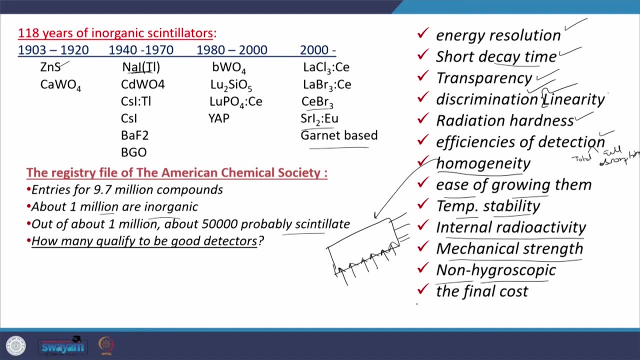 So the second parameter is the cost. So the third parameter is the cost of the nuclear reaction. ok, So how good it is in terms of mechanical strength, whether it is hygroscopic or non-hygroscopic. If it is hygroscopic you have to encase in some aluminum kind of caning. 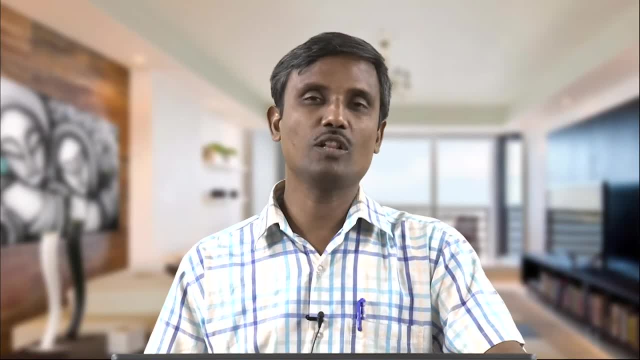 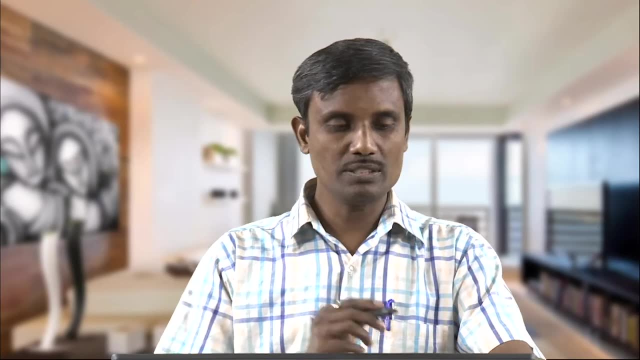 ok, And then, of course, the final cost. So all these parameters comes into picture when we decide any scintillation detector. ok, Let me give you one simple example regarding the energy resolution, which is the first property I mentioned in the previous slide. 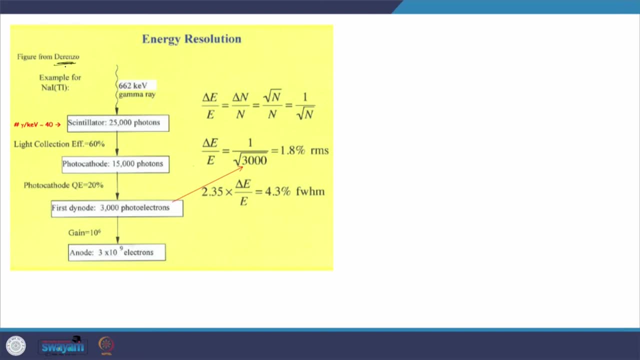 So it has been taken from the notes of Derenzo So you can see here example for the sodium iodide: if you take So 6 is to keV gamma ray. if you consider it will emit 25000 photons. considering 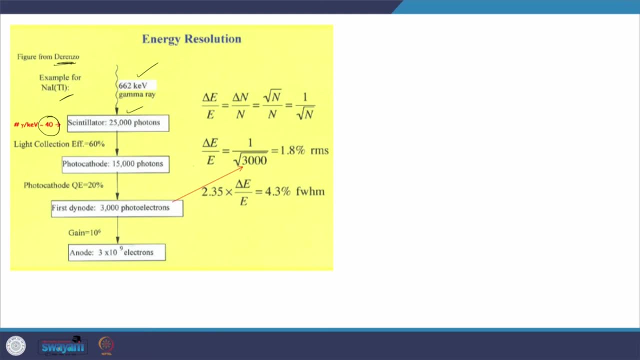 the per keV ok 40 number. if you consider, and if the light collection efficiency is 60%, then so many photons will reach the photocathode And the photocathode quantum efficiency. if it is 20%, then are emitted 3000. and considering that gain of the PMT as 10 to power of 6, then at the 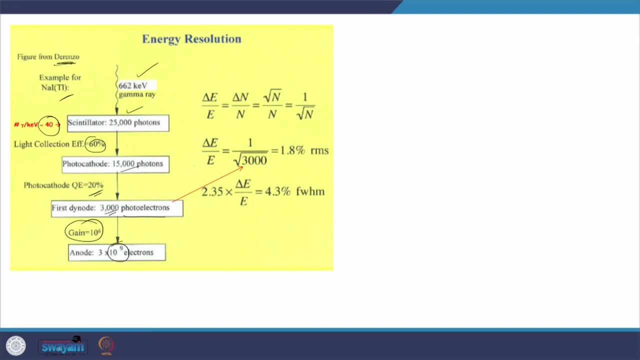 anode, you are getting 10 to power of 9 electrons. ok, And here this 1 by square root of n 3000 is giving rise to delta E. by E and multiplying with 2.35, you are getting 4.3 percent of. 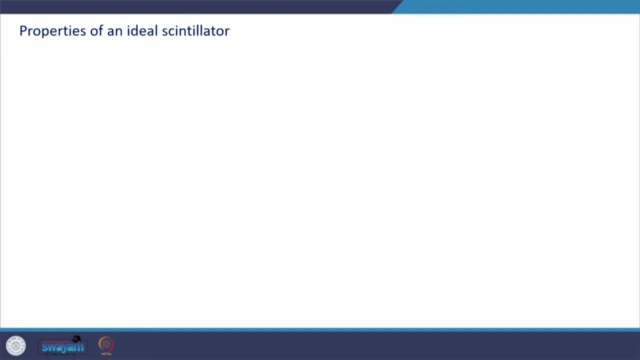 full width at half maximum. alright, And what are the properties of an ideal scintillator? It should be able to convert the incident energy into detectable light with high scintillation efficiency And, as I said, linearity yield and incident energy of wide range should be. 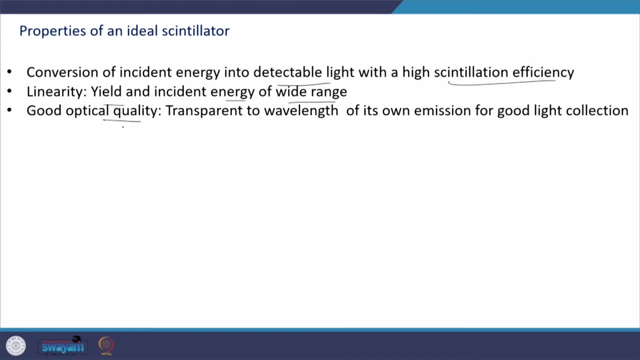 linearly rated, and optical quality should be very good. Otherwise, whatever optical photons are created, they will be absorbed within the crystal, and one should be able to grow in large sizes. Decay time also should be very less. The refractive index should be in such a way that it should be matching with the glass. 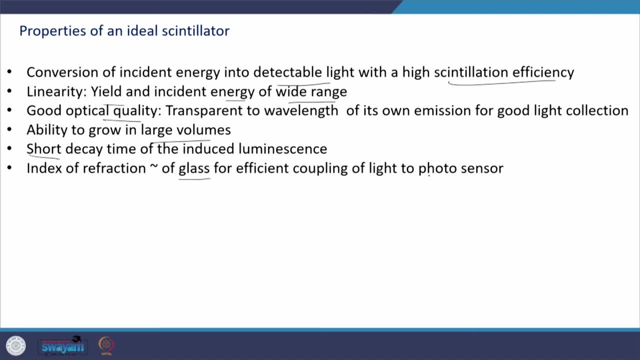 So that it should be in such a way that it should be matching with the glass So that coupling can be efficient when we couple the scintillation crystal to the photosensor, And fluorescence should be maximum and minimum delayed fluorescence and phosphorescence should 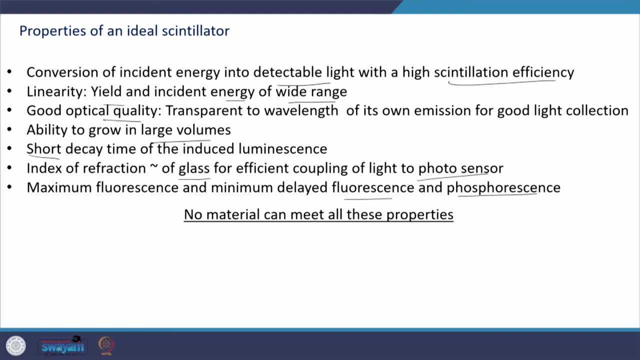 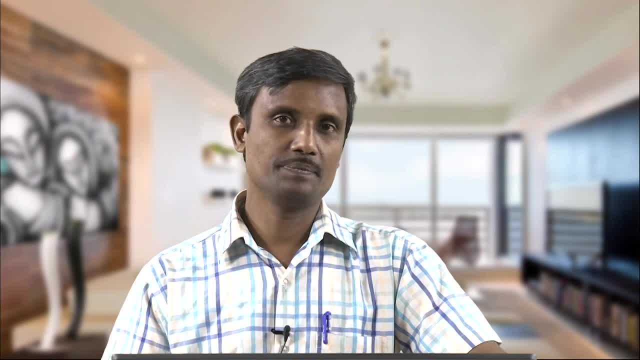 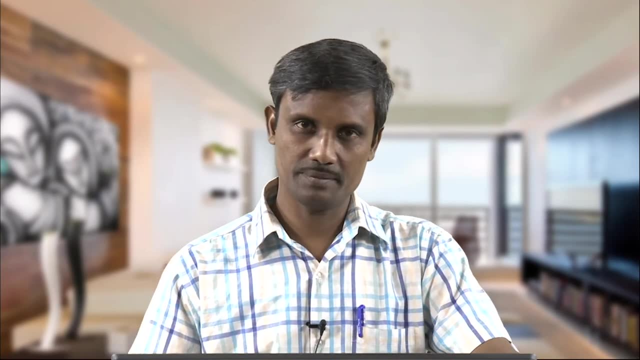 be very less ok And of course, there is no material which can satisfy all these properties. So there is a tradeoff between the properties and, depending on the application and available resources, one should choose the scintillation detector, All right. And if we consider inorganic, they are best in terms of light output and linearity. 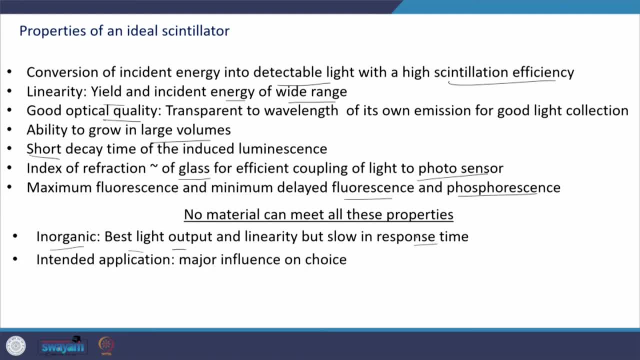 But the problem is they are not very fast. ok, So the intended application decides the major influence on the choice. choice, ok. And for gamma spectroscopy, mainly we prefer inorganic detectors. Of course we also use the semiconductor detector. And when we use inorganic detectors, 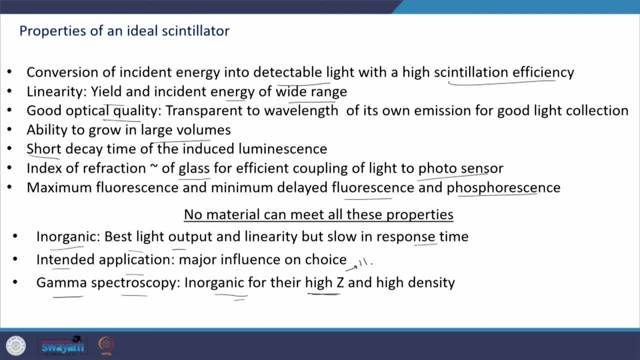 the main reason is for high Z, which gives rise to high Z, So we prefer inorganic detectors. So these are the two effects of the high Z detector. So high Z detector is defined as high detection, efficiency of detection and the high density. 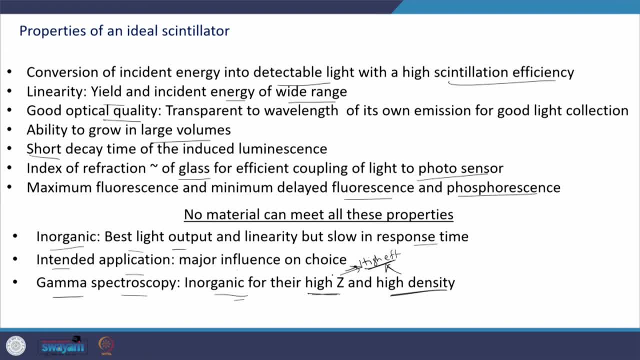 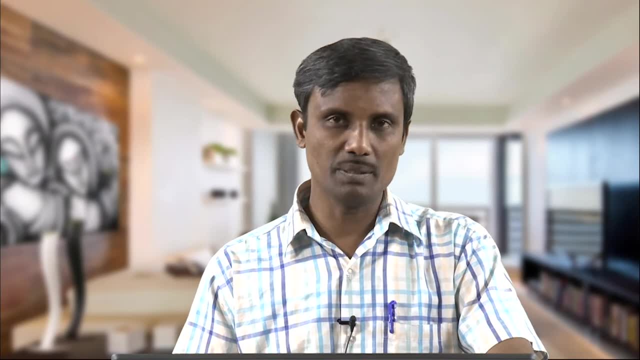 and high atomic Z. they lead to the high detection efficiency. All right, and for normally, for detecting the beta and fast neutrons we use the organic Because, considering the nature of interaction of beta and neutrons, we prefer the organic molecules, which normally contains. 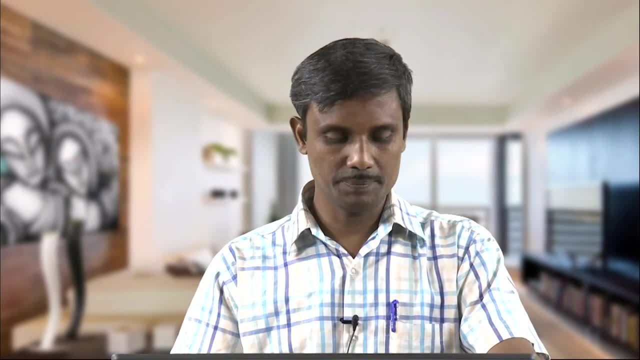 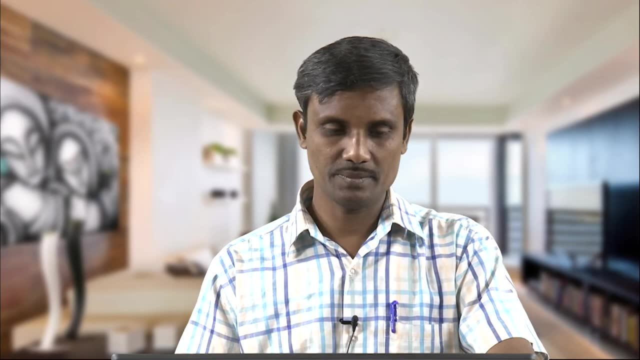 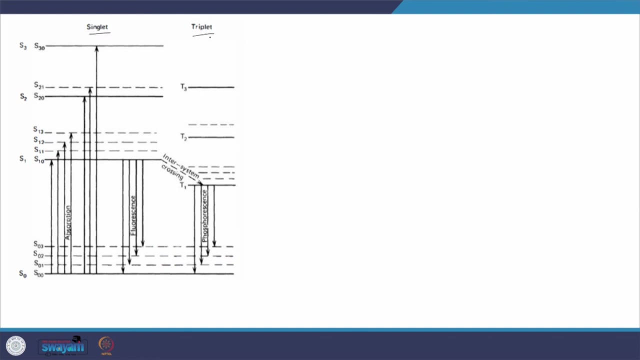 hydrocarbons And the reaction. the interaction of the, this neutrons, with the hydrocarbons leads to better nuclear reaction probability. alright, And this is how organic scintillator works. You have singlet states and triplet states, The transition after following the excitation which gives us the fluorescence. ok, So it. 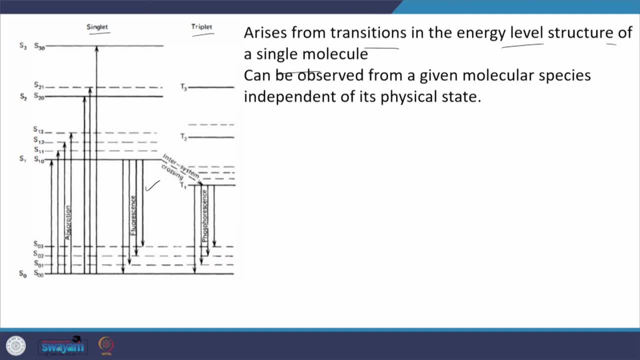 arises from the transitions in the energy layer structure of the single molecule and it can be observed from the given molecular species, which is independence of its physical state. That is the interesting point in the case of organic scintillators, And it has so called pi electron structure And the net effect of this transition is the population. 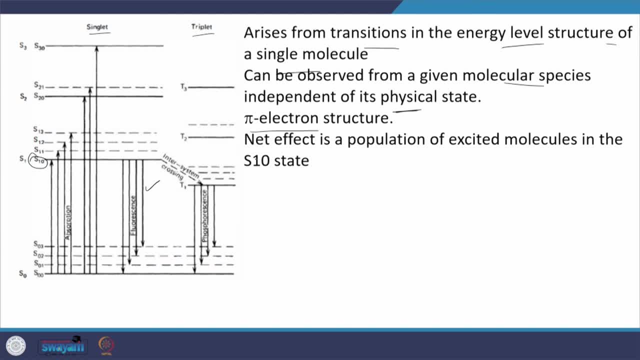 of exited molecules in the S 10 state. This is the S 10 state. ok, So this is basically S 10 state. You can see the transitions are taking place mainly from here only, ok, And while in the T 1 state some molecules may be thermally exited back to the S 1 state.